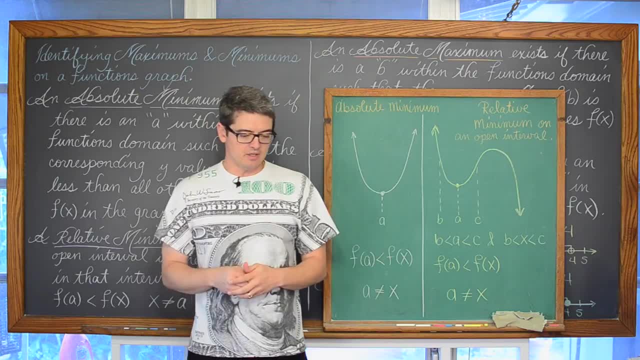 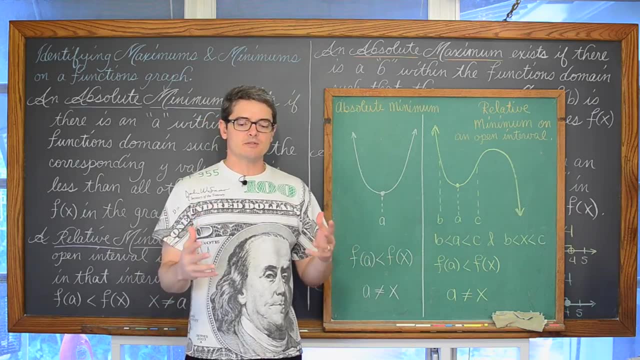 to earn off of a new idea or product that you are developing. There are a lot of real life applications, but in this example, this lesson we are going to be just looking at, five graphs that are given to us not necessarily applied to some kind of real life setting. 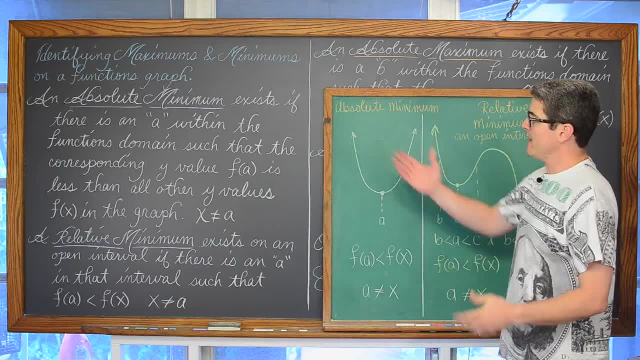 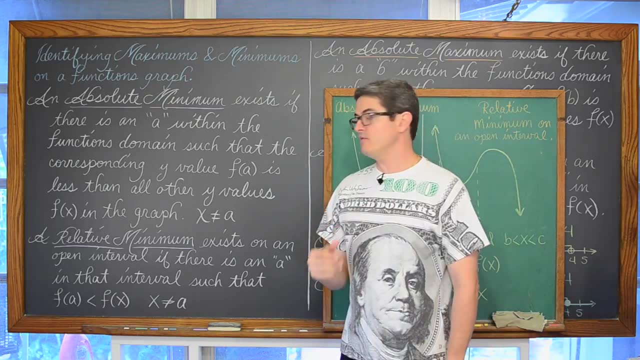 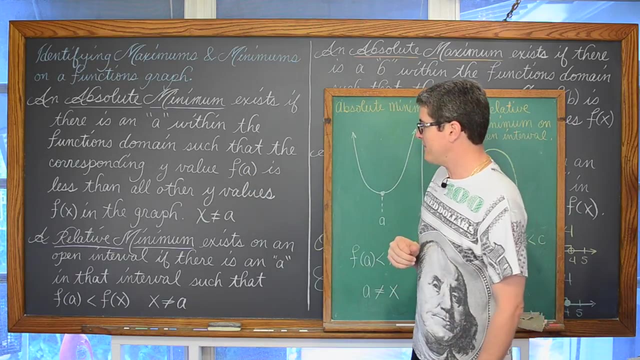 Identifying maximum and minimums on a functions graph. Well, an absolute minimum exists if there is an a within the function domain, Such that the corresponding value of y written as f of a, because we are using function notation- is less than all other y values f of x in the graph where x is not equal to a. That 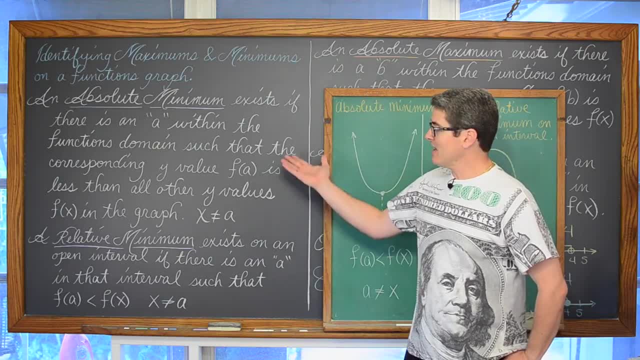 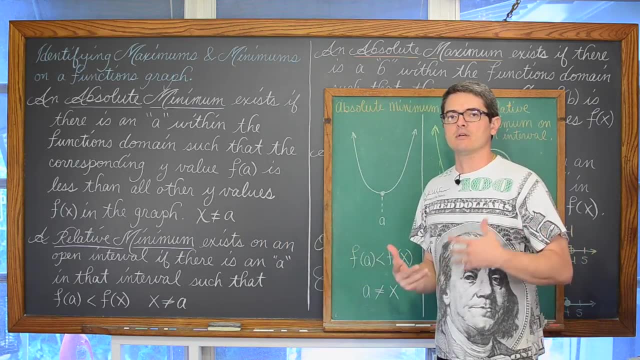 sounds very mathy, and well it is, And there is a lot of good vocabulary words in here that we do need to know and understand through our studies of mathematics. so we know what the teachers are asking us to do for a particular question, or we can follow the directions in 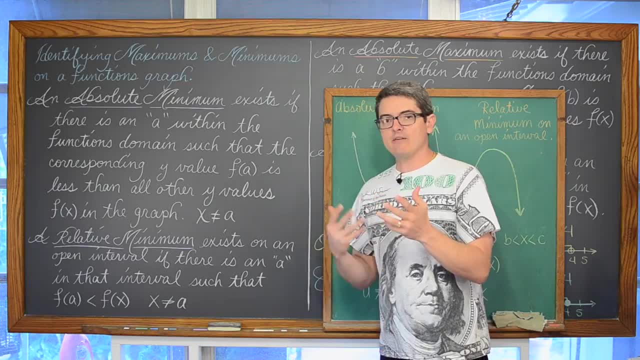 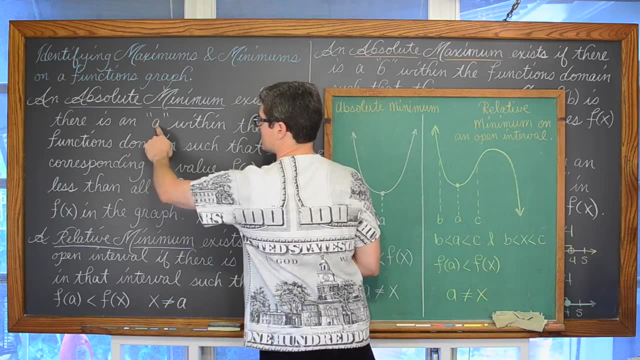 the textbook, But just in case you haven't been watching all of my algebra videos in sequence, we have a value of a. Well, within that sentence it says value of a is within the domain of your function. We will write the domain as your input values. and if you are just talking, 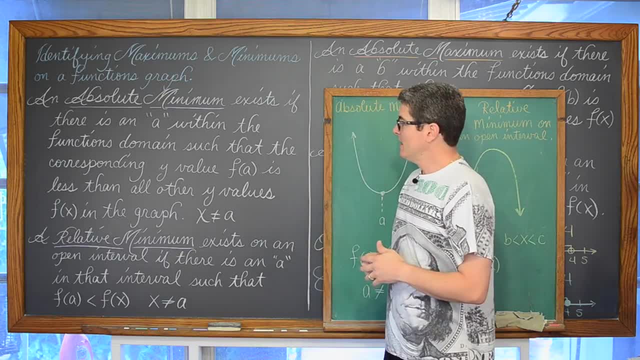 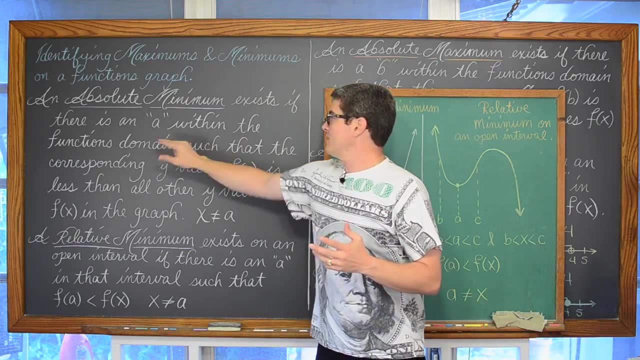 about a graph on an xy axis. they are the x values. So a within the domain. that is part of the sentence that is telling you that this is an x value, That there is an x within the domain, Such that the corresponding y value will. 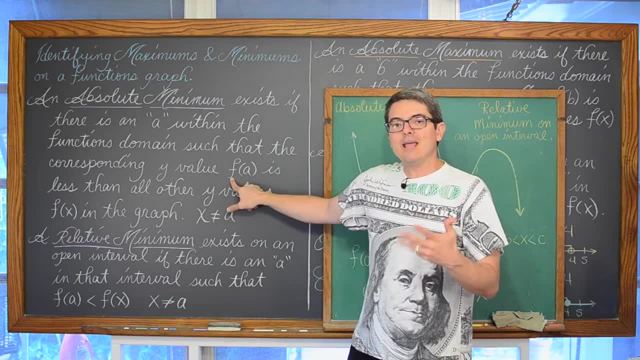 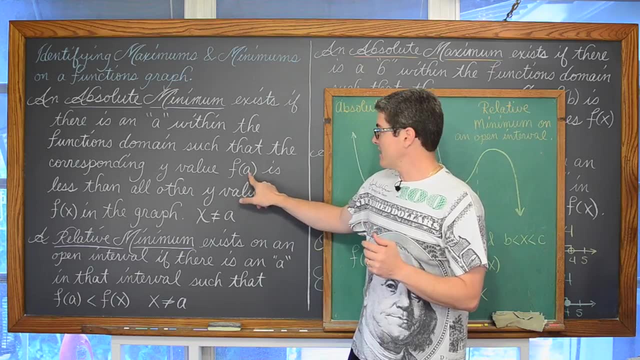 f of a. that is where f is the name of the function. this is function notation and the variable that is inside the parentheses is the independent variable, the x. You plug in the x, the input value, you get out the y. We can name the horizontal and vertical. 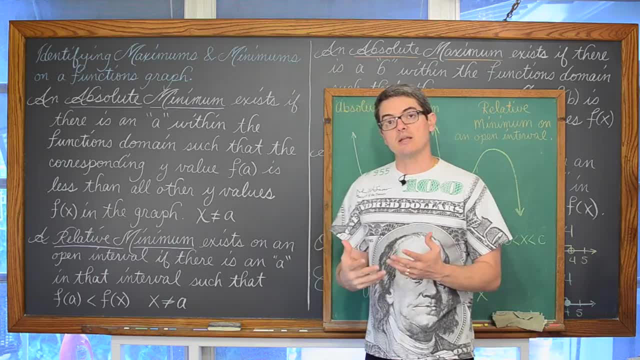 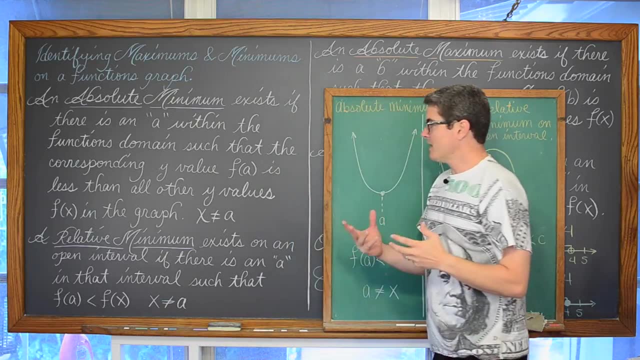 axis with other variables, if we are talking about some kind of application setting, word problem setting. but you know Cartesian Plane is x and y axis, So x and y is less than So. this value of f of a is the name of the function. this is function notation and the variable that is inside the parentheses is the independent variable. the x: You plug in the x. the x value: you get out. the x. You plug in the x value. the x value: you get out the x value. and the variable that is inside the parentheses: 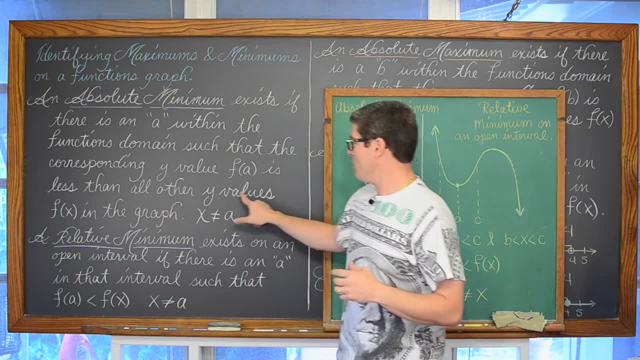 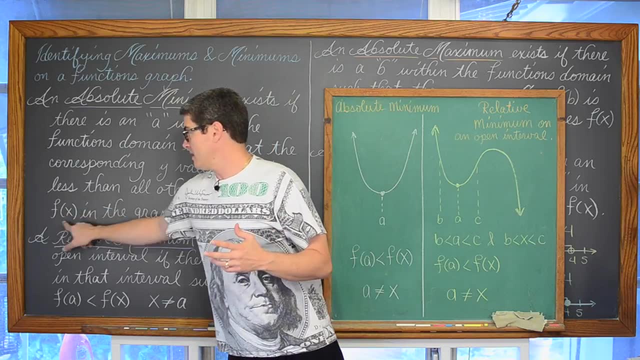 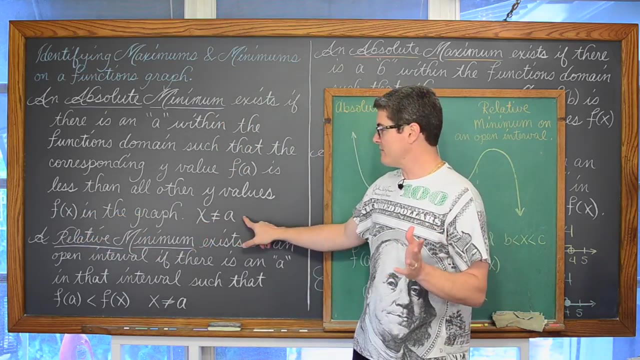 So f of a is giving some kind of y value and that y value is less than all the other y values. and this f of x means just any value of x within the domain That you are getting some value of y, That this y is less than this y over the entire graph, Except for when. 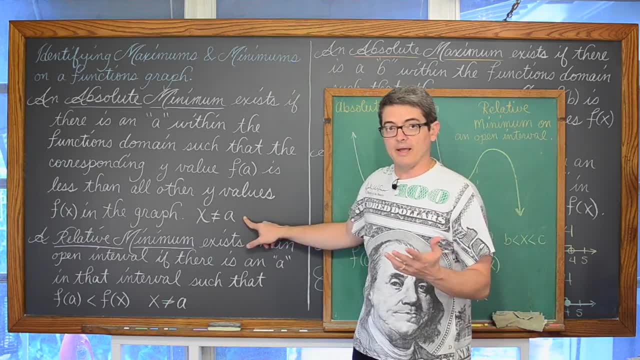 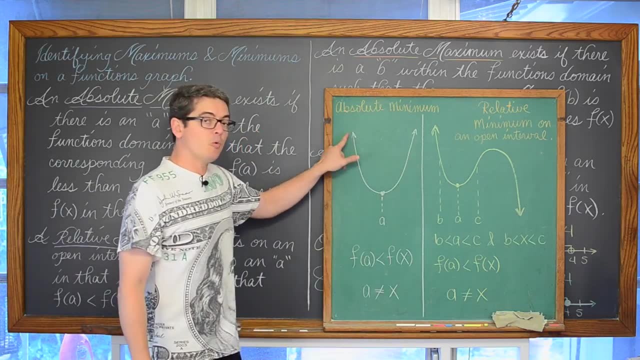 x is not equal to a. You know, everywhere x is not equal to a. Because, well, to put it into a picture, so you kind of understand what I am talking about, here we have a parabola, parabola that's opening up. Now, because this parabola opens up, there's one point, that's: 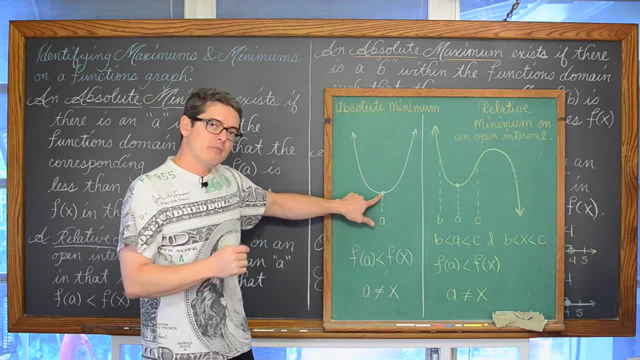 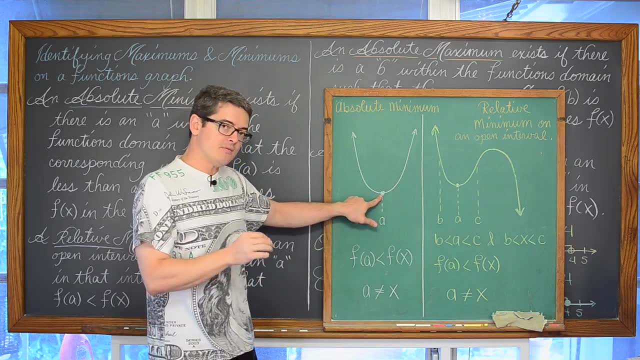 at the very bottom of that dip. Well, at the bottom of that dip, that's going to give us our smallest y value. Remember, the y values are the up and down movement. There's some point at the bottom that gives us the smallest y value. that's included throughout this entire. 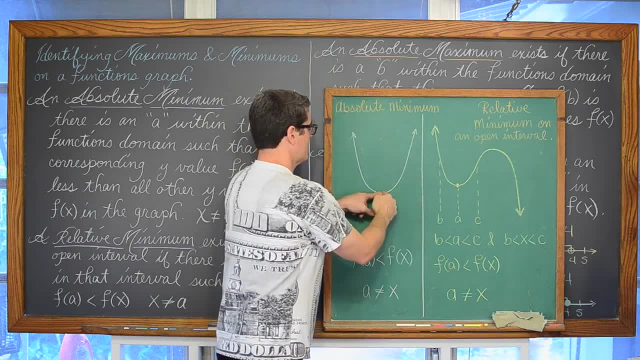 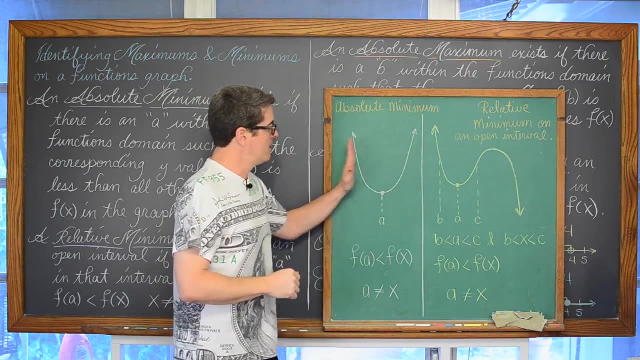 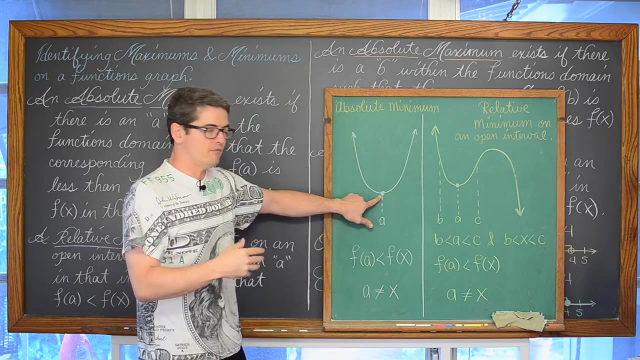 domain of this graph, because from this point, the vertex, the graph opens up in both directions, So that y value is the lowest, the smallest y value within this entire domain. So that point, that vertex, if you haven't studied thoroughly your parabolas yet, this is just. 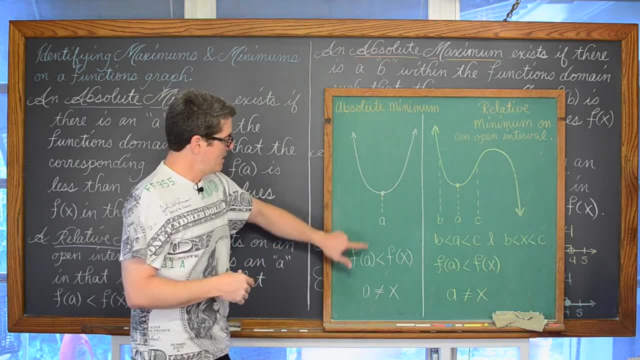 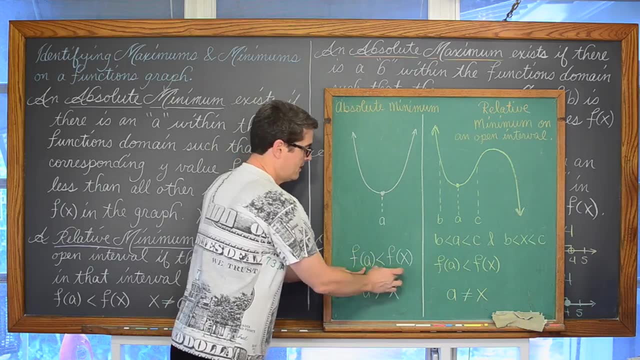 for purposes of pointing out what an absolute minimum is. but for that value of a, that x value of a, f of a, the y value of that point is less than the y value that you're going to get from plugging in any other value of a. 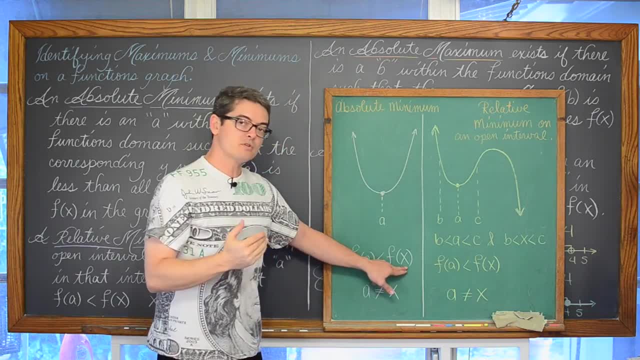 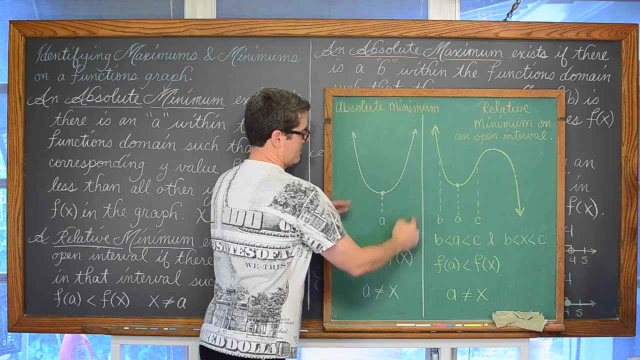 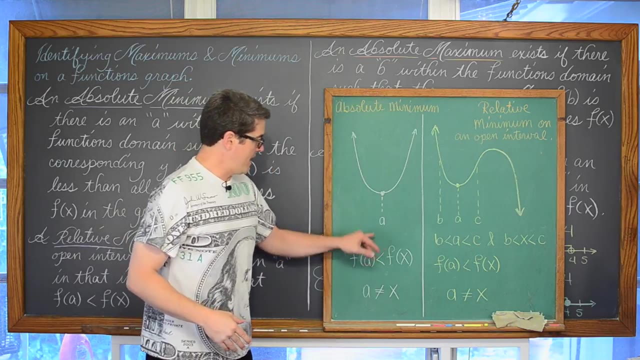 x within the domain right, And of course domain is again that horizontal movement along the x axis or any x value that you can plug into the function and get some kind of real output. And if a was equal to x, since a is an x coordinate, if a and x were representing 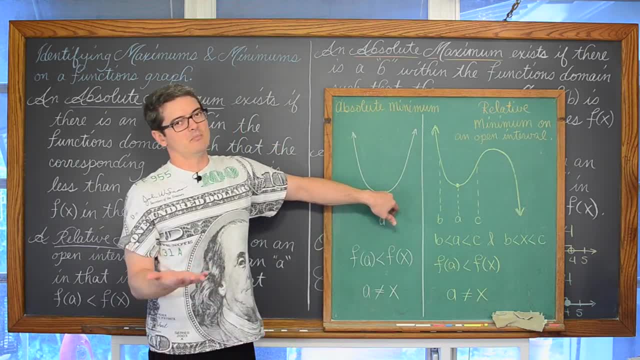 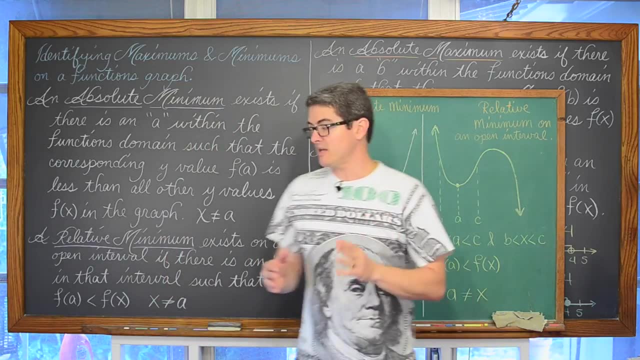 the same numerical value and they can't because they're different letters. you'd be looking at the same point, right? And we're looking for that absolute minimum, The absolute lowest y value. that's included within the graph. So I hope that makes sense. 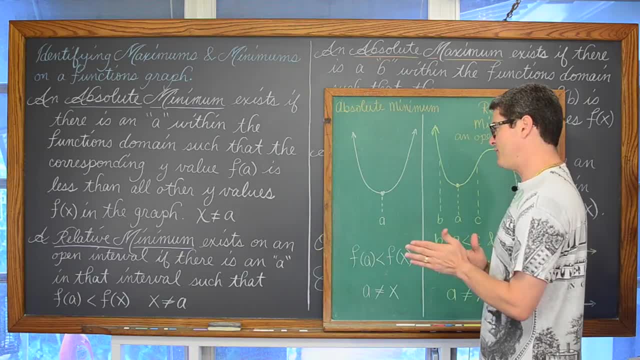 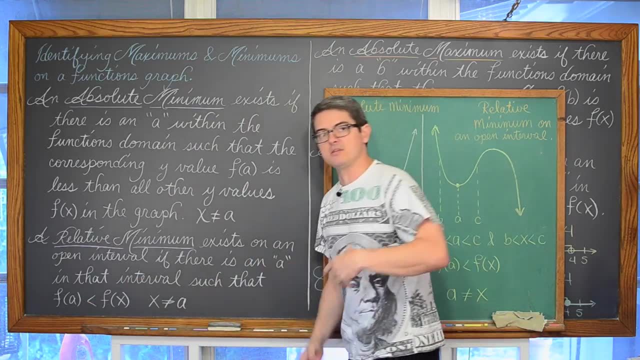 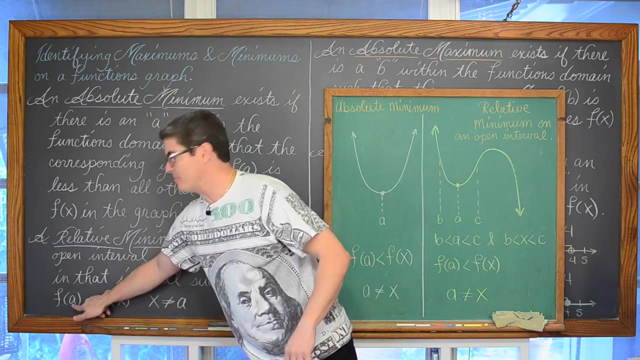 A relative minimum exists on an open interval if there is an a in that interval, such that again f of a and we see the a again in the parenthesis. so it's still an x value that, the y value that we get the whole f of a expression, that y value that we get by plugging. 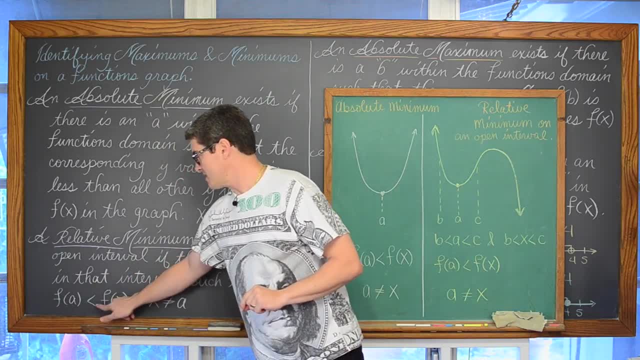 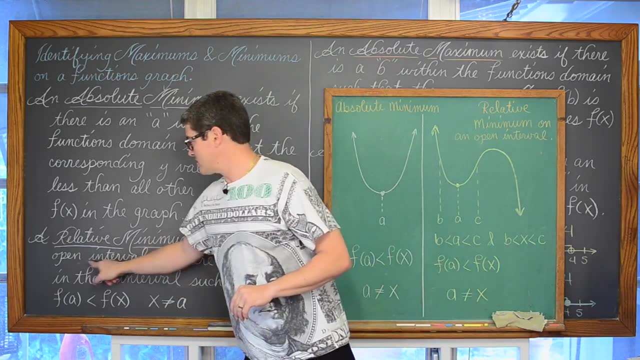 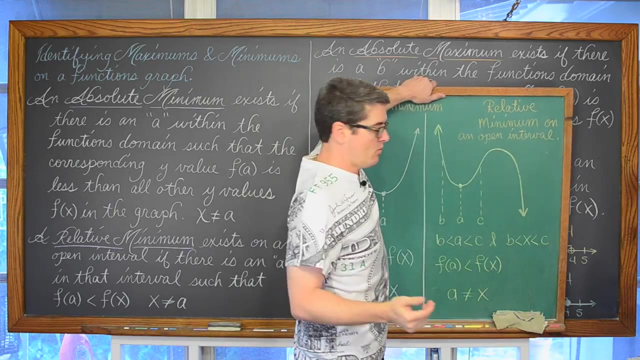 that particular value of x into the function is less than the values of y we get from plugging any other x Within that function, that's, in this open interval. Okay, well, maybe you have either not learned or have forgotten what an open and closed interval is, So let me get this. 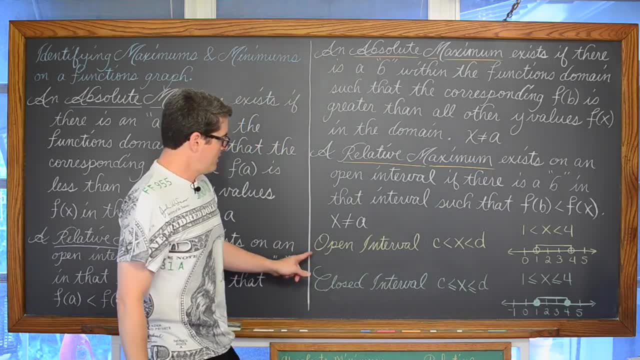 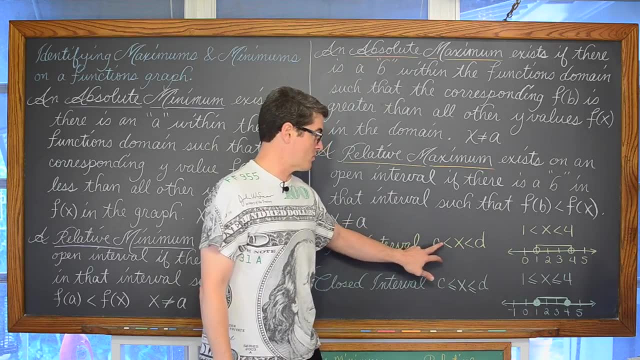 out of the way. Remember graphing inequalities on a number line. An open interval is some kind of example where we have- in this case, I have written that c is less than x, or x is greater than c, And then that x is also less than d. So, uh, to put it that way, I 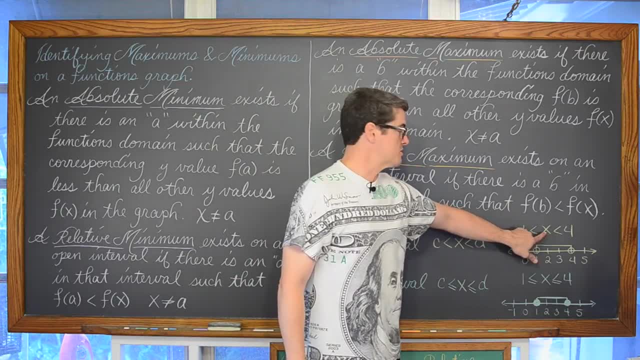 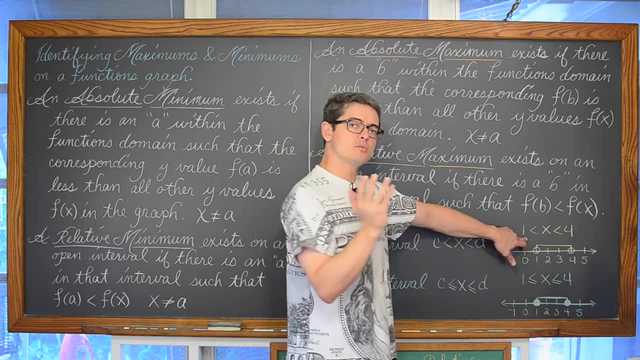 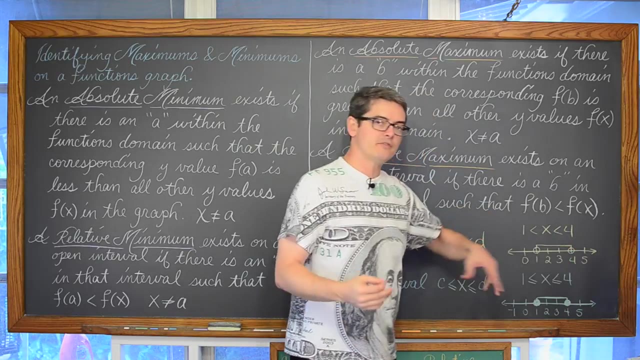 put some numbers to it. Here's an open interval. Here's an x which is greater than one and less than four. So any value of x that's just a little bit bigger than one- like 1.0000001, would be good, And any value that we can put in for x that is less than four, even if it's. 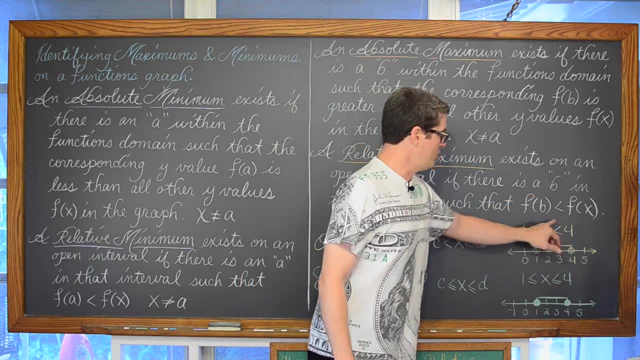 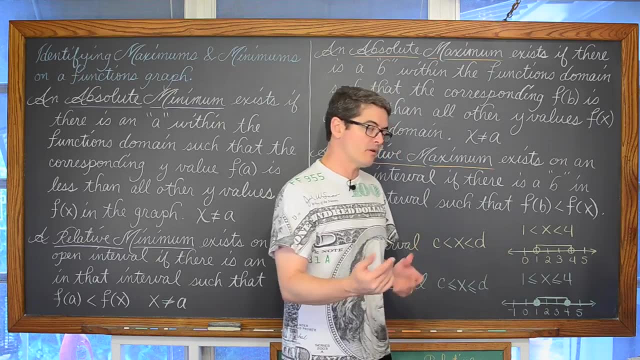 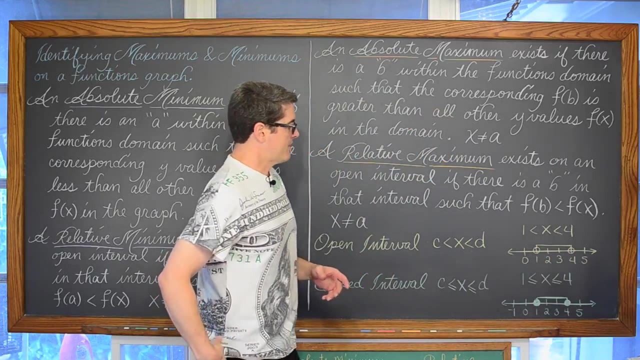 three, point nanananana. Any value, any numerical value between one and four is a solution, if you will, to this open sentence. So to graph it on a number line, you put an open dot on one, an open dot on four and shade between those open dots. Now that means that 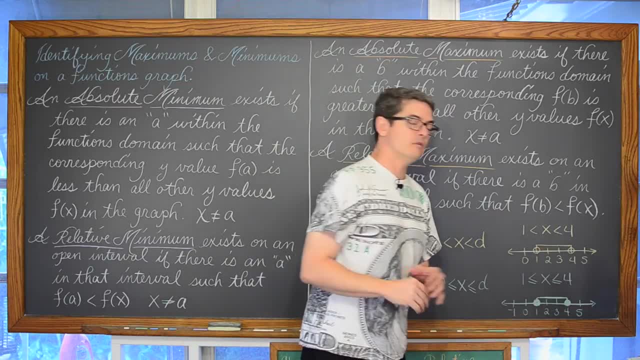 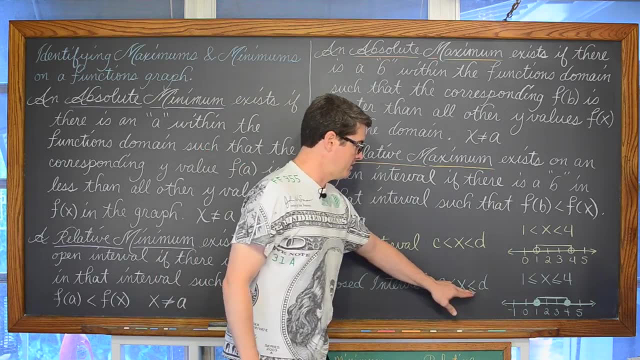 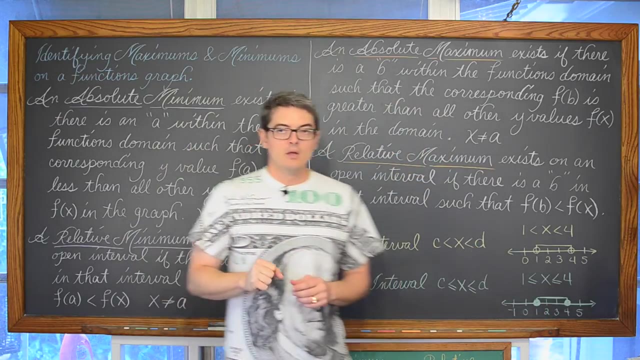 the value of one is not included in this interval, and nor is the value of four. It's an open interval. A closed interval is when you include the end point- See the equal signs here now- And when I graph it on the number line, those dots are closed. So when we're talking about 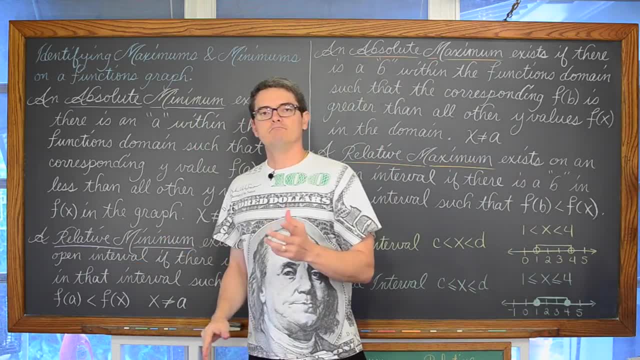 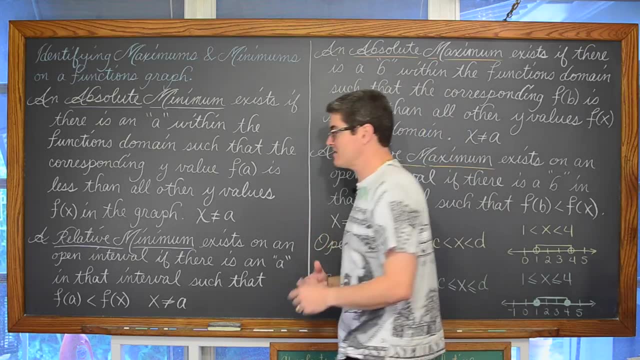 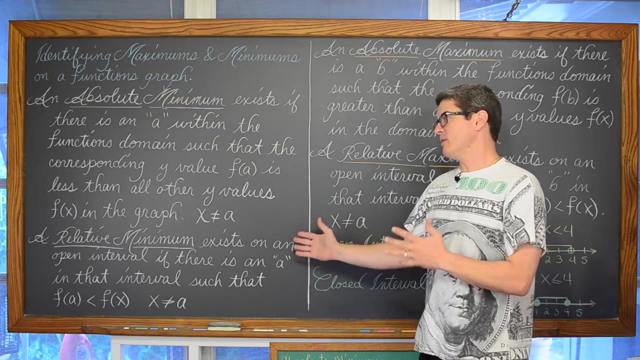 exists on an open interval. you know well. Let me get the phone Alrighty, then, And I'll be pointing out the importance of paying attention to this idea of open and closed interval as we go through the examples that are in this lesson, And it might seem like a little bit of a technicality in this definition. 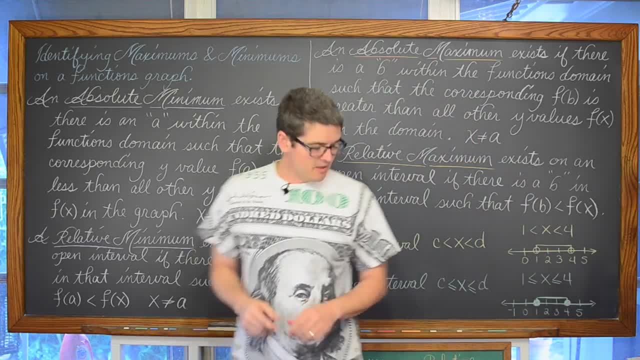 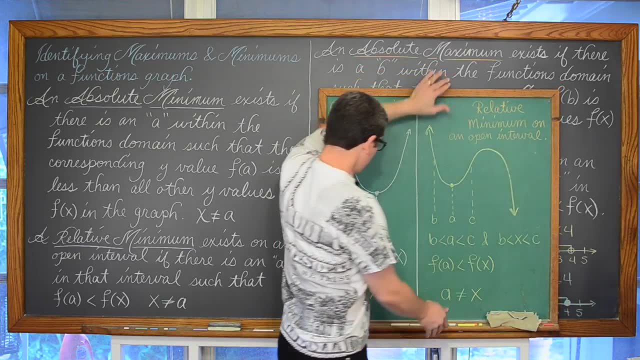 but it does have it's point where you do need to pay attention to it. Now getting this drawing back up here: my pitcher in pitch-a- very high tech. we've already discussed how this parabola that was opening up had an active interval. Now I'm going to go back here and 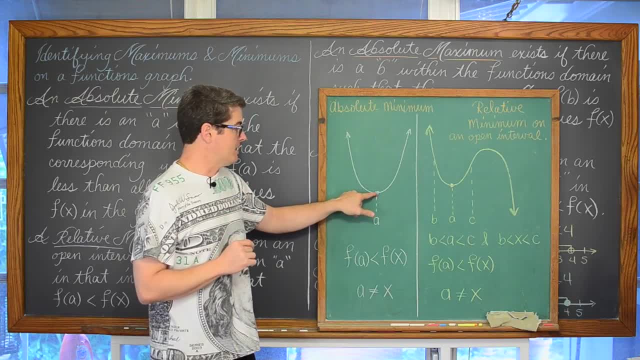 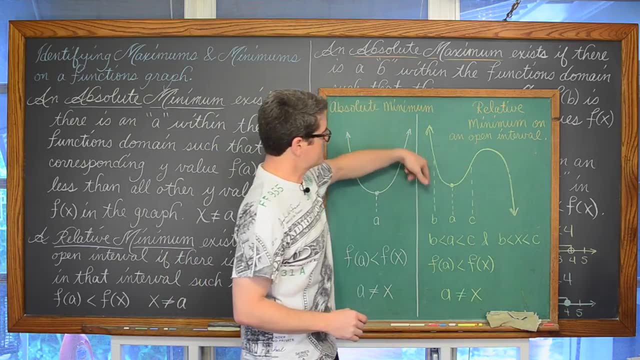 do an absolute minimum. There's just one point on this graph that has the lowest possible y-value, So there is an absolute minimum here. And now we have kind of what's looking like a cubic function and it goes up forever and it goes down forever. So the fact that it 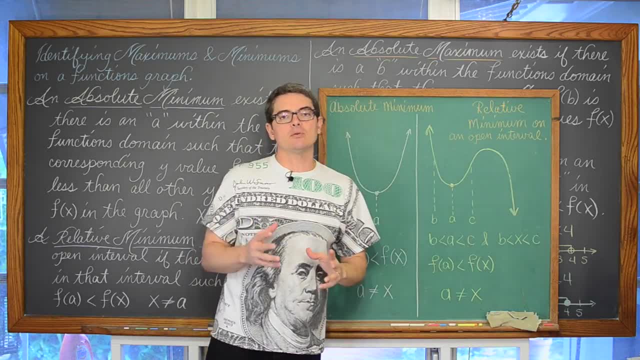 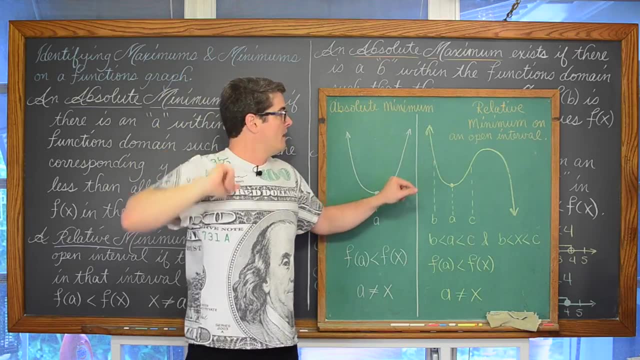 goes up forever means that that graph has no absolute maximum. It just keeps going up and up and up. And as soon as you say some y-value that you think is the greatest, well it's just going to go up a little bit higher And it also goes down forever. So that graph 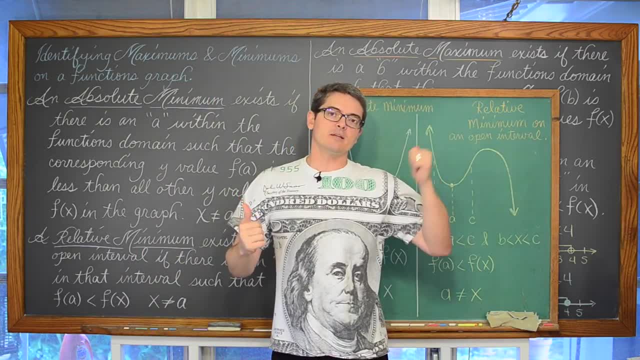 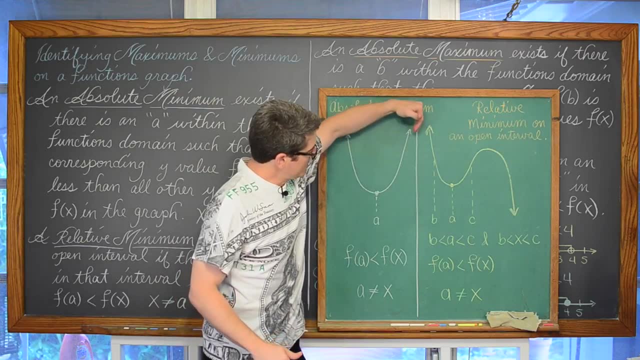 does not have an absolute minimum and I haven't defined it, but it doesn't have an absolute maximum yet either. I'll go a little bit faster on the second half of these board notes. But it does kind of, as you read it, left to right, it kind of does dip down and there's a bottom. 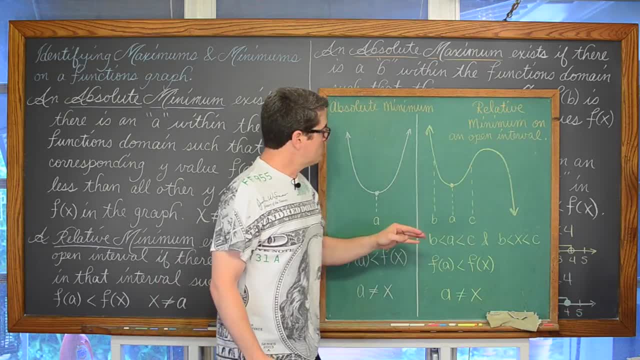 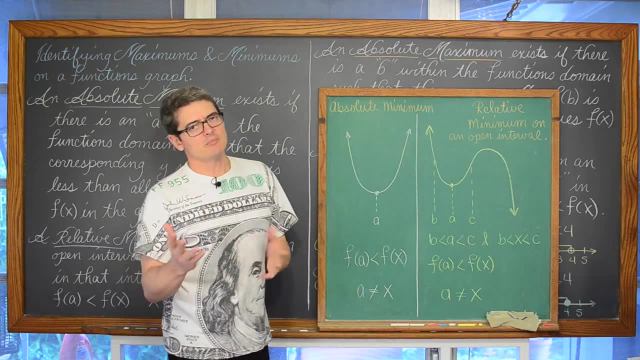 there. It kind of looks like the one that's over here And then it rises back up again. So it does fall and then start to rise again. And this cubic function I know in Algebra 1- maybe you haven't been exposed to cubic functions yet, but it does have a domain of. 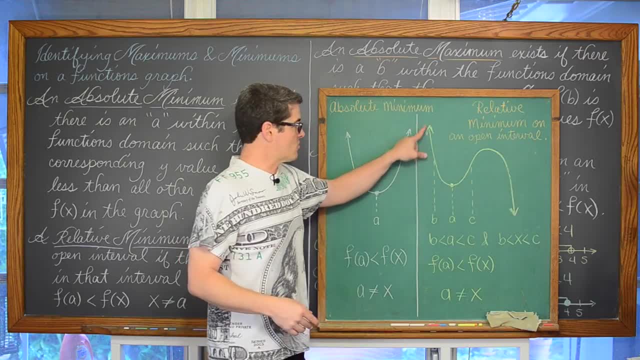 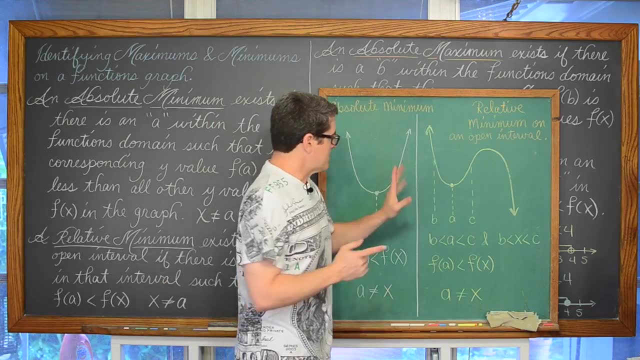 all real numbers, So I can draw the entire graph without ever picking up my pencil. A little bit of a preview of a definition of continuity there, But okay. so there's some kind of open interval from b to a And remember, these are x values. So there's an x value here and there's an. 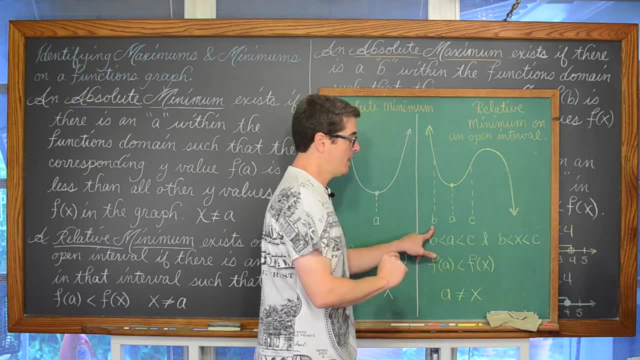 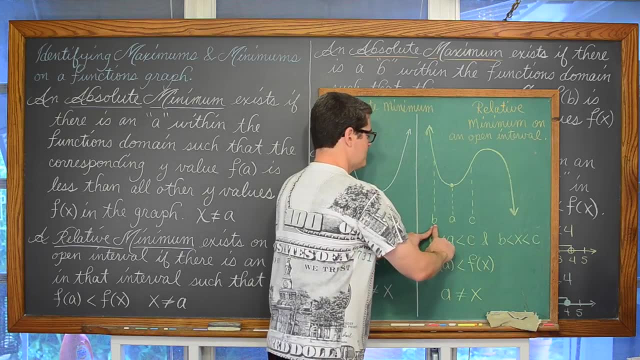 x value here And a is somewhere within that open interval. And now for this notation, we also need to assume that x is within that open interval as well. So within this interval from b to c, this open interval from b to c, a is greater than b and less than b. And 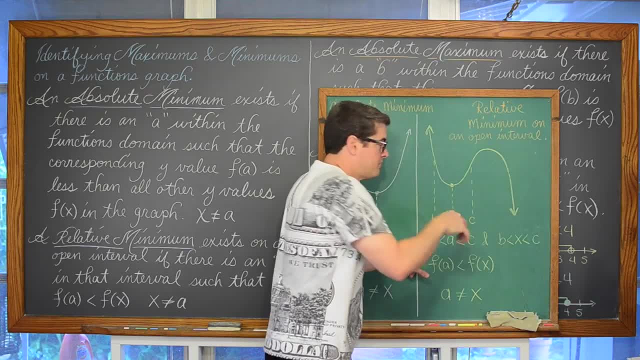 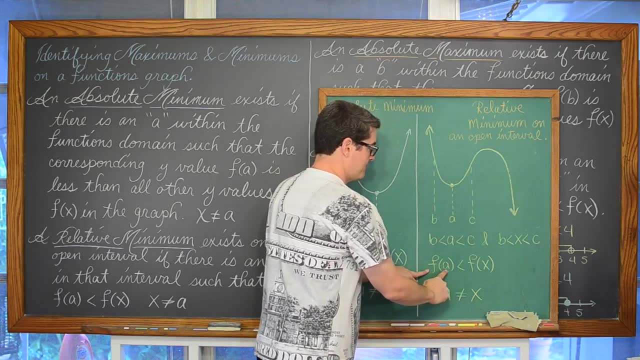 b and c. There is that bottom point. We can see it So mathematically, all math-y talk, that means that f of a, within this open interval, there is an f of a, there is a y value that. 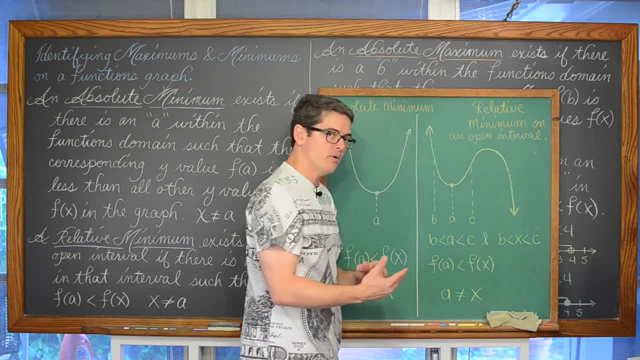 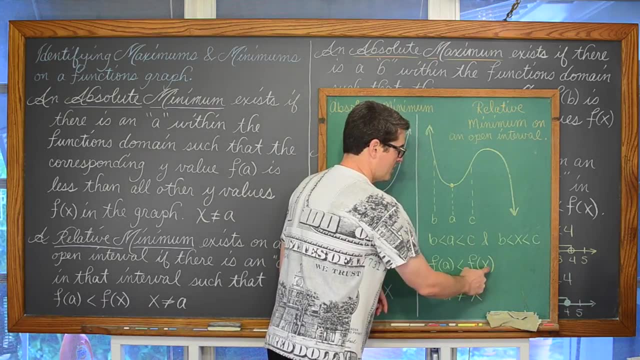 you get from plugging a, that x value, into the function, You get some kind of y value that is going to be less than smaller than all the y values that you get when you plug- well, all the other y values that you get when you plug x's in between b and c, All those. 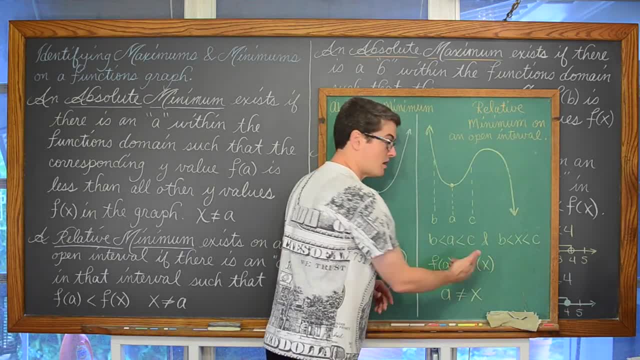 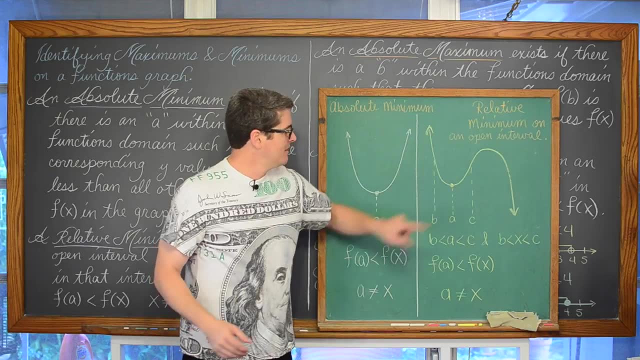 values. when you plug in any other value of x on this open interval, That y is going to be smaller than that y, Again assuming a is not equal to x, because then you are talking about the same point. So absolute minimum and relative minimum. Graphically we are going. 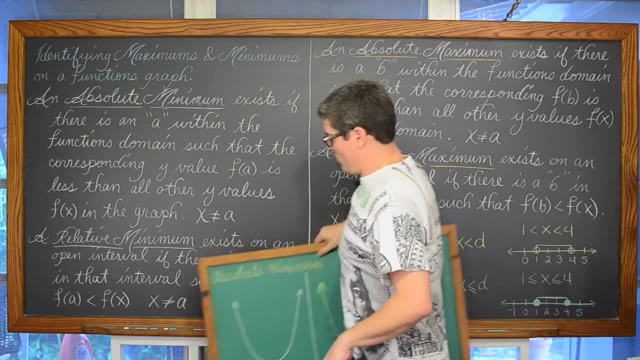 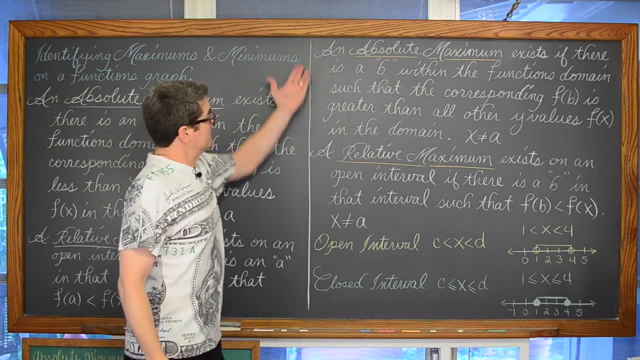 to do a bunch of examples, but this is such mathy language. I thought that would help you to hopefully understand these definitions. Now this half is going to be much quicker, because it is just the opposite. An absolute maximum exists if there is a- b within a function's. 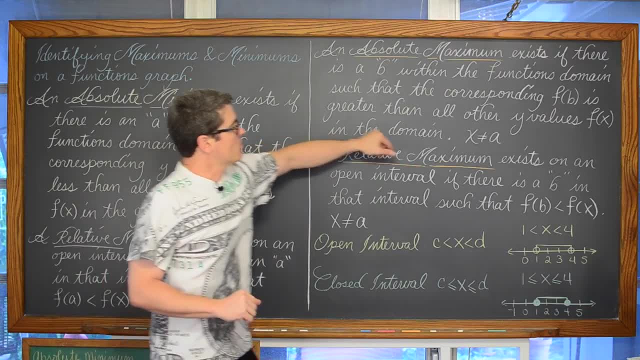 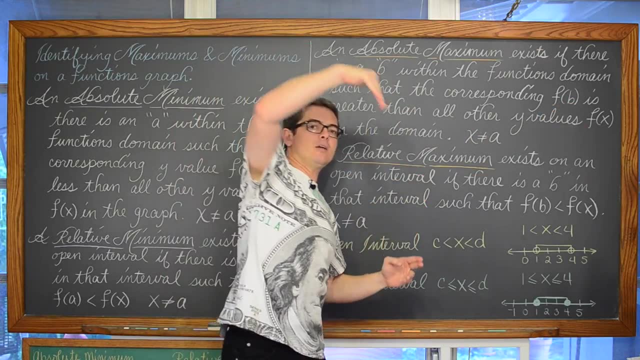 domain within all the possible x values, such that the corresponding f of b- again a y value that you get when you plug in b- is greater than We are talking about a maximum value, and then the graph starts to fall: again Greater than all the other y values. f of x, If you. 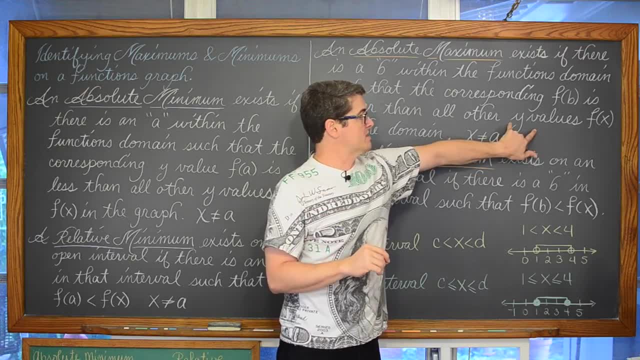 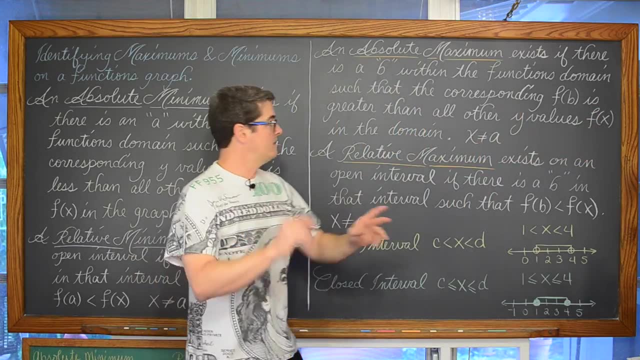 really understand function notation. I am being a little bit redundant in how I am writing this sentence because you should know, if you understand function notation, that that is a y's. But I am telling you twice, basically in the same sentence, that, hey, that means y in the. 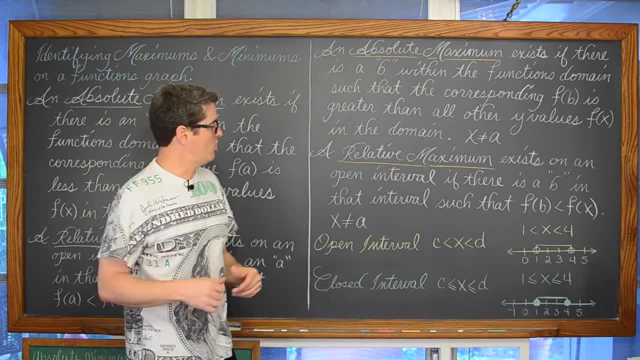 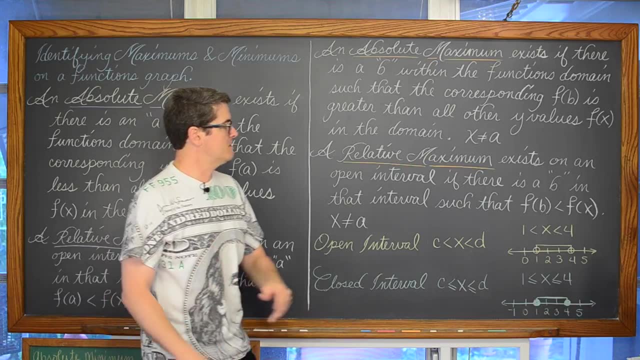 domain where again x is not equal to a, because then that would be the same point: A relative maximum. a relative maximum, not an absolute maximum, exists on an open interval if there is a, b in that interval, such that f of b see the b again inside the parenthesis. so 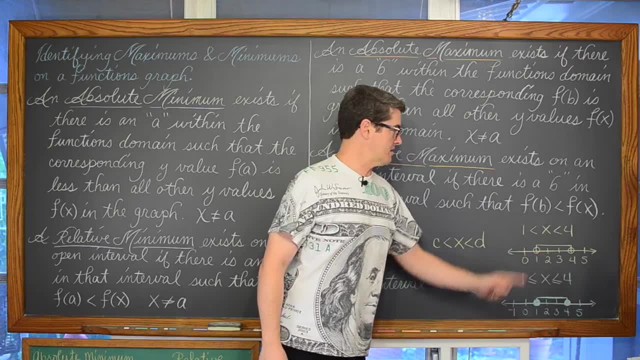 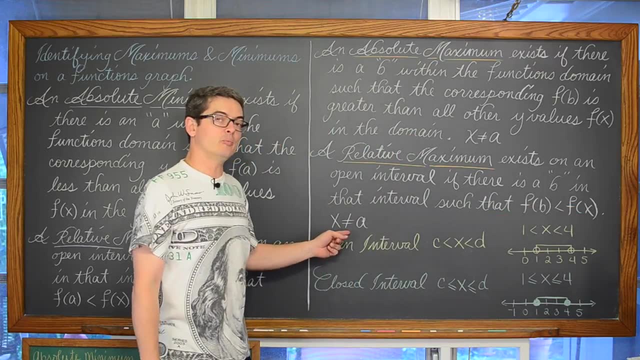 it is an x value, that f of b is less than f of x. This y is less than that y, Any other y that you can possibly get, Any other x on that open interval, assuming x is not equal to a. Ok, so that is all the. 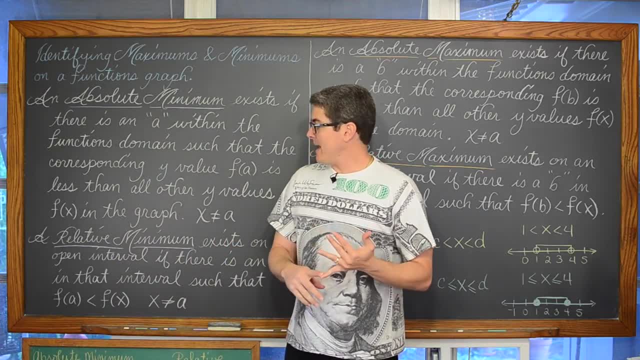 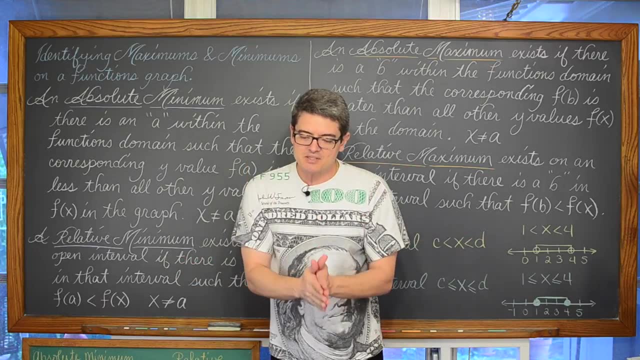 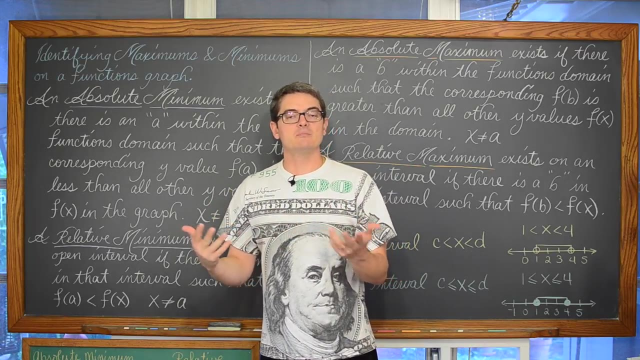 formal math language of definitions for absolute max and min and relative max and min, Except I am saying that in reverse as I am pointing to it, So lets get one at a time. We are going to take a look at 5 graphs and identify the absolute and relative max and min of those. 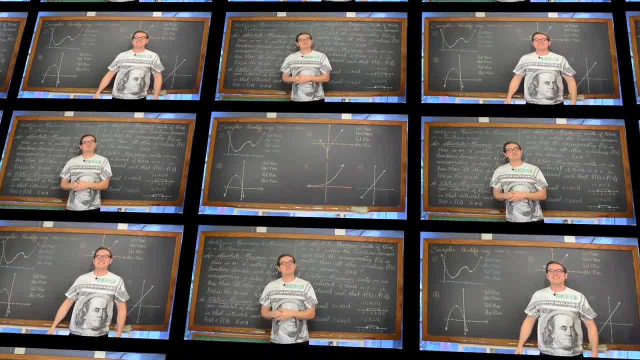 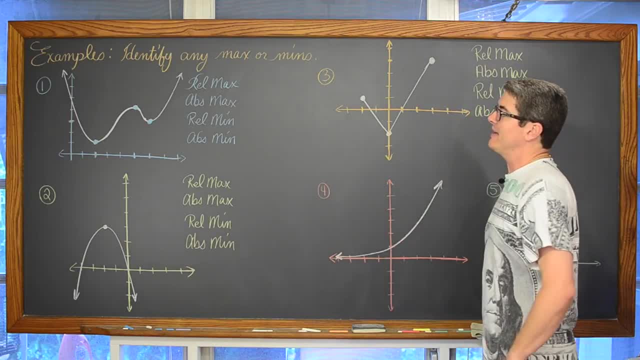 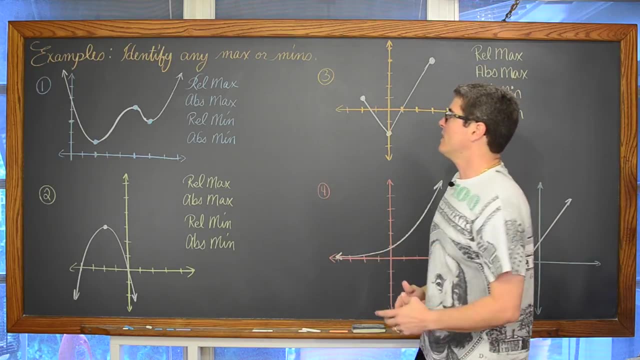 graphs if we can. No, no, no. So here we have our five graphs. We are going to identify any maximum or minimums, whether they are relative or absolute, for each of these graphs. We have sort of a weird thing here. We have a graph that is rising to the left and rising to the right, with a few dips. 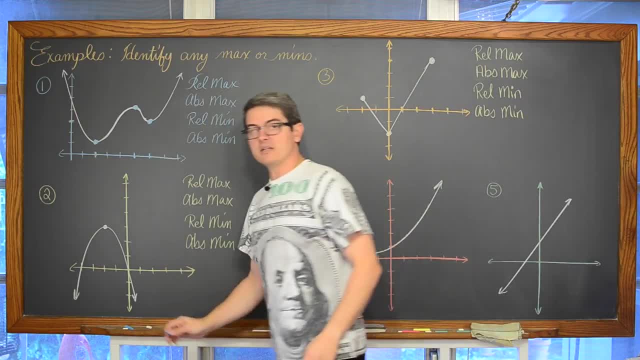 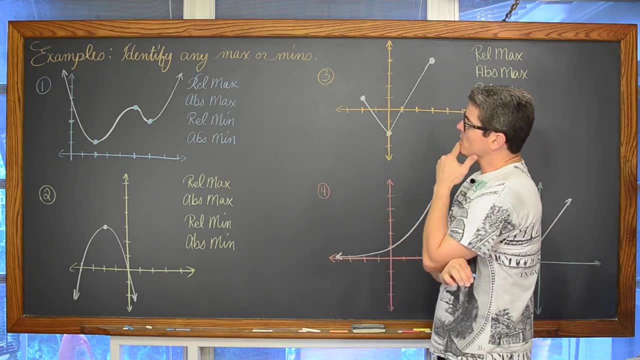 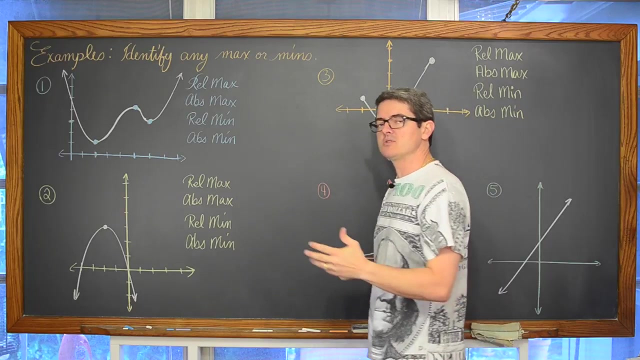 in the middle. We may learn later in our algebra studies that that looks like a polynomial to the fourth degree, Graphing higher order polynomials, And we are going to find a relative max, if there is one. Is there an open interval? Is there a place within that graph that you 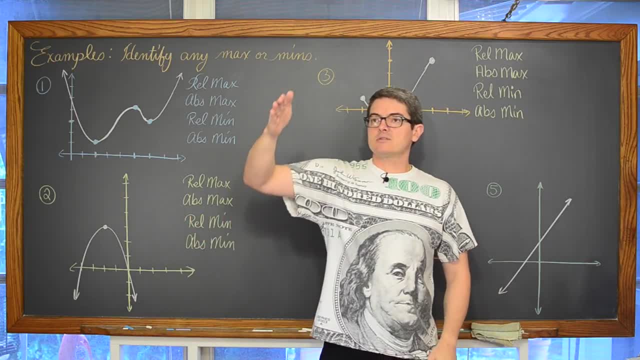 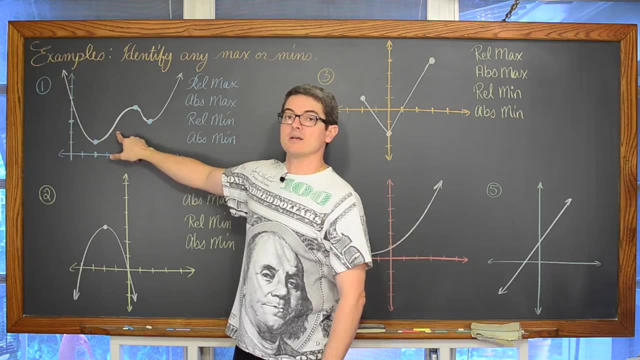 see where it kind of, as you read it left to right, that it kind of rises and then falls. Well, it is falling here and it dips down. It looks like it is going to be some kind of minimum, because it starts to rise up again. Remember when we are looking for relative. 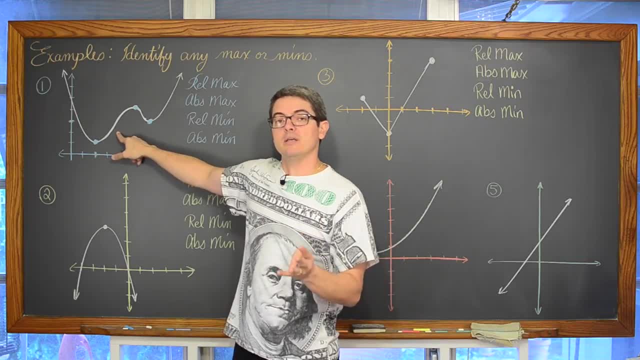 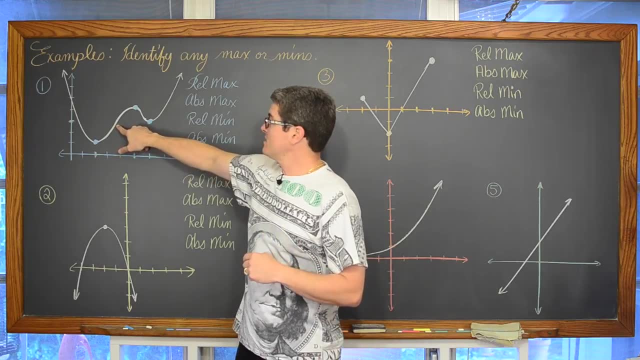 max or well, forget the word relative. When we are looking for max and mens, we are looking for y values. What is a high or low y value? The y values are increasing because the graph is rising to the right. Then we get to this blue dot and it starts to fall again. So it seems like somewhere. 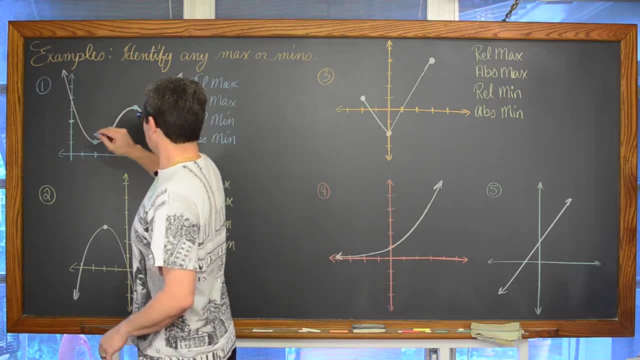 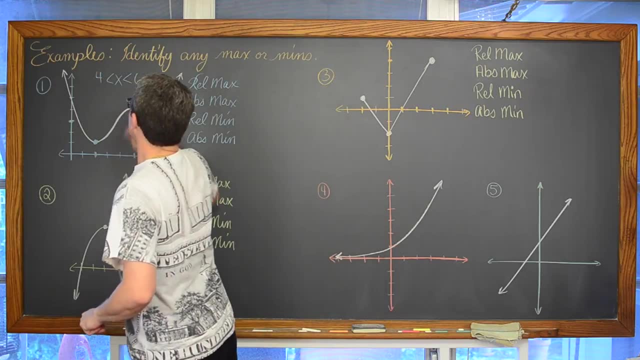 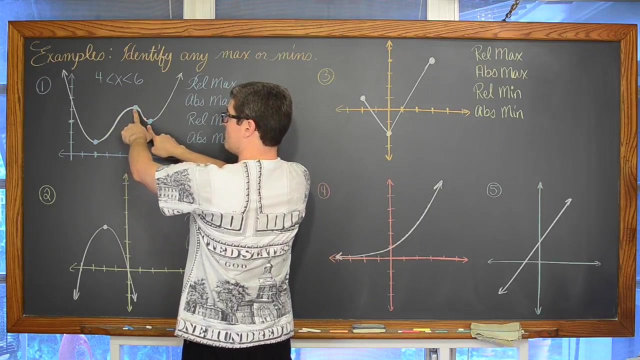 here maybe an open interval from where x is greater than 4 to 6.. Within that interval from 4 to 6, if I look at there, the graph is rising and then it starts to fall again. So it looks like that we do have a relative maximum there. Now we have a relative max of 1,, 2,. 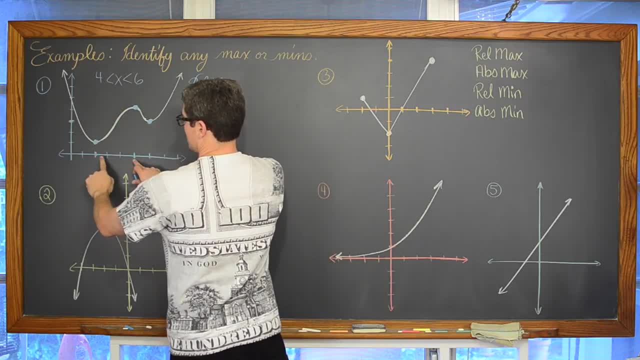 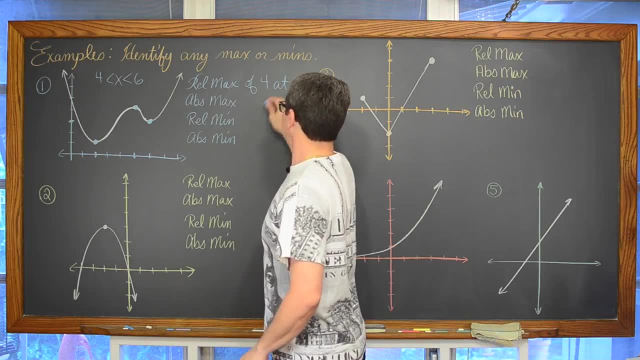 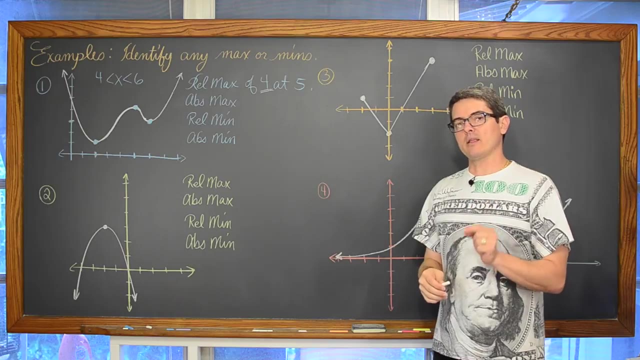 3, 4. 5.. So we have a relative max of 4 at 5.. Now identifying the max and mens is about the y value. but I like to also identify where that y value is at. So we do have a relative. 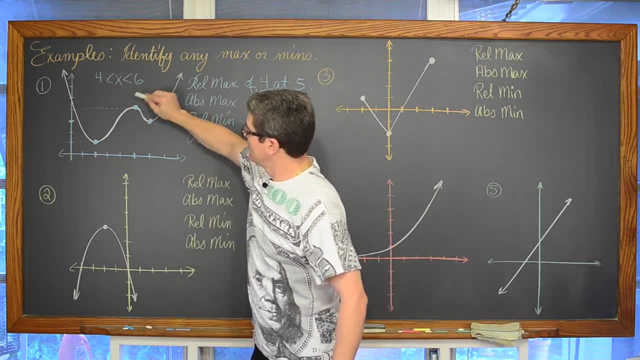 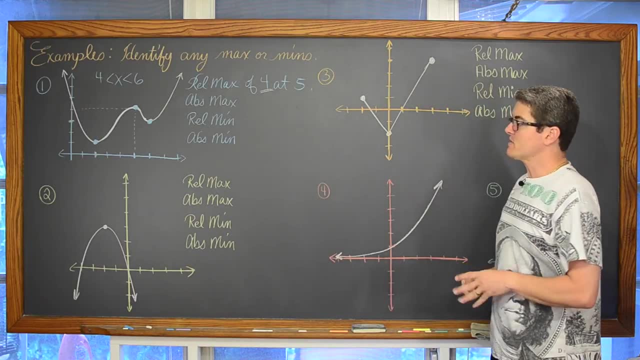 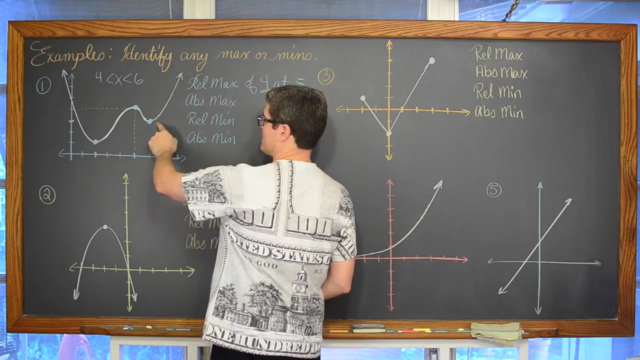 max again of 4 at the x value of 5.. The maximum is the 4.. Now is there an absolute maximum? well, we do reach and high point here and the graph starts to fall. But then it starts to rise up again, and on both sides, to the left, and 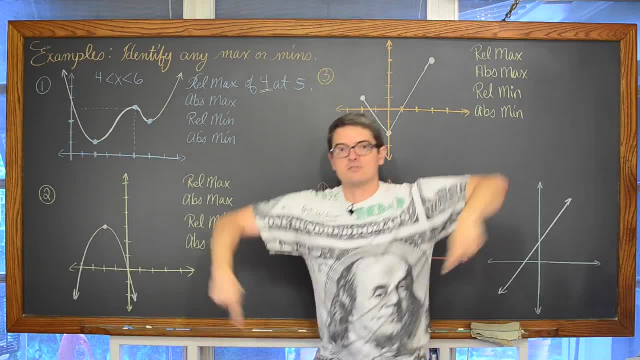 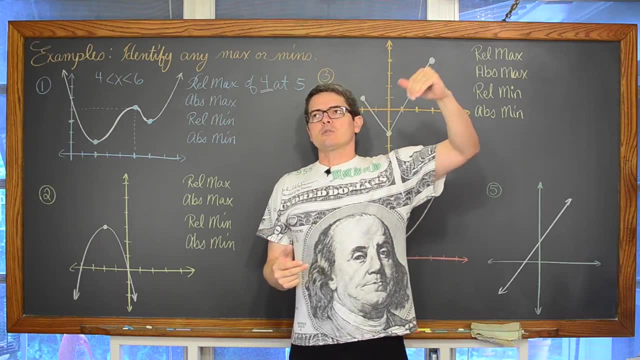 to the right as x decreases and as x increases, that graph starts to shoot up and those arrows mean that it never stops going up. So there is never going to be a real y value, which is the greatest, because as soon as you see it is like a million. then I can keep going. 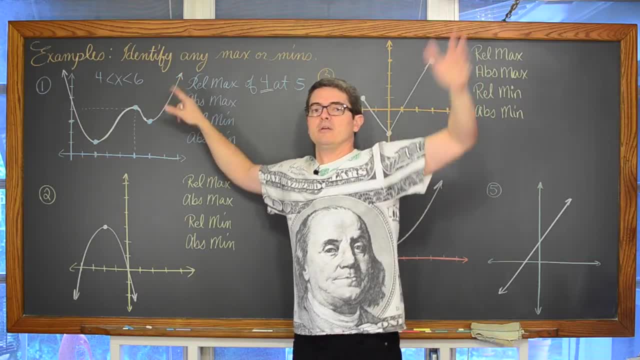 up. Don't just say: oh no, it is a million and a 1.N And a million and 2 and a million and 1.. There is no real value, but there is a absolutely absolute maximum in the graph: itsحد and a million and two, a million and three or a trillion, a billion, a zillion, whatever. 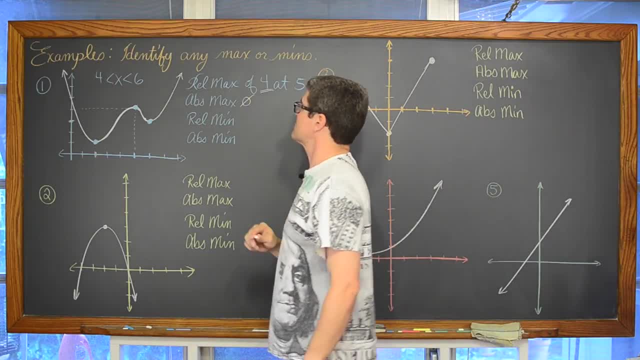 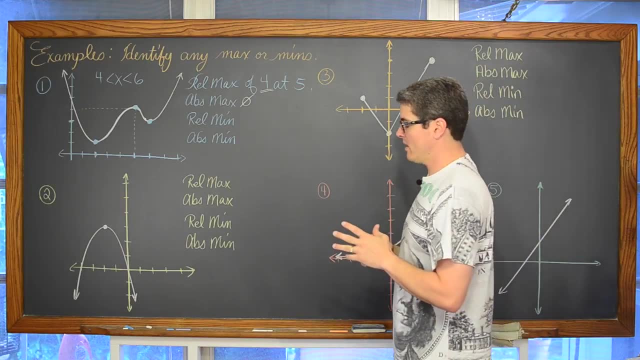 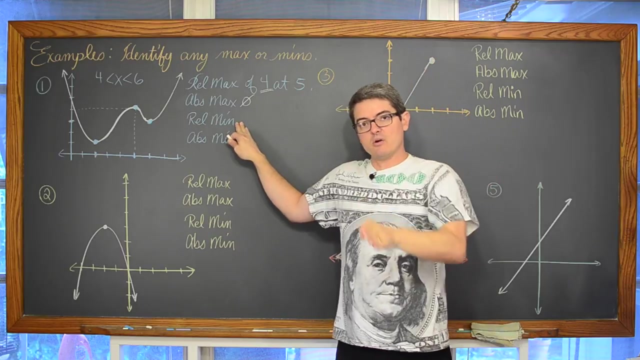 There is no absolute maximum value. Is there a relative min? Again, is there some kind of open interval where the graph has a minimum value, where, as you read it, left to right, the graph is dropping and then it starts to rise again. It can be a sharp bend or it can be. 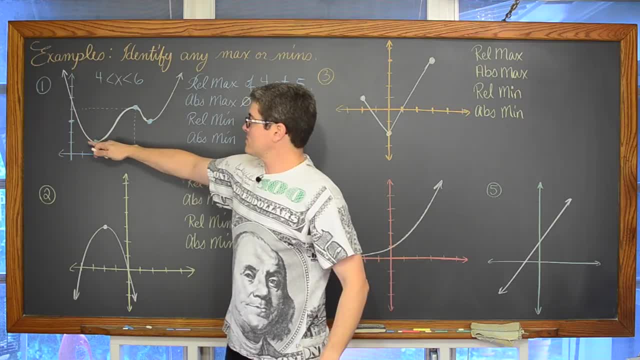 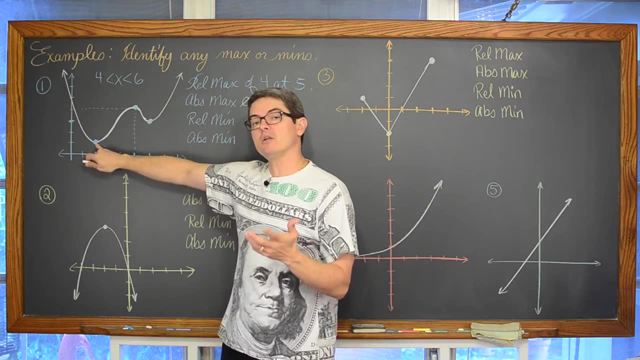 a smooth curve. Well, it is falling to the right and then starts to rise again. so it seems like at that x value of two we have a small or the smallest y value that exists, and it starts to rise up again and then it starts to fall again. So there is actually 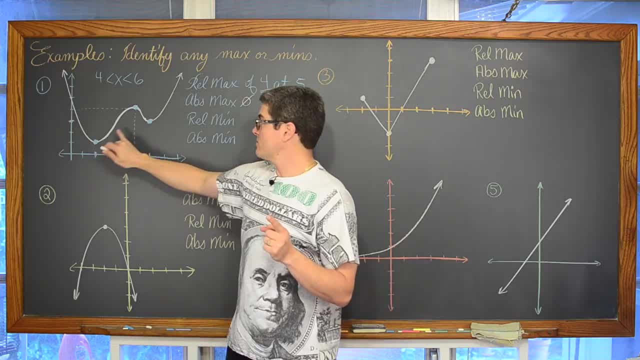 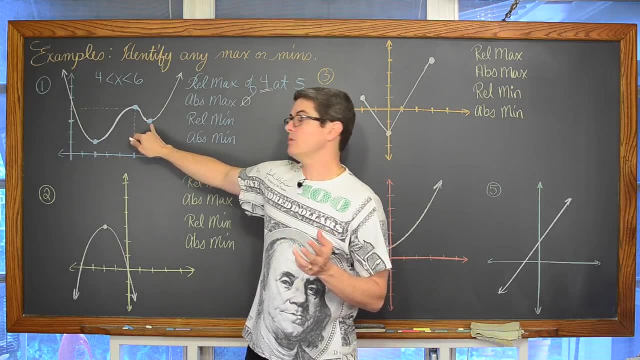 two minimums. There is a minimum y value of one and there is a minimum y value of. looks like I tried to make it about a y value of three. Well, one is less than three, So the one is going to be an absolute min for that entire, you know, and the absolute mins are: 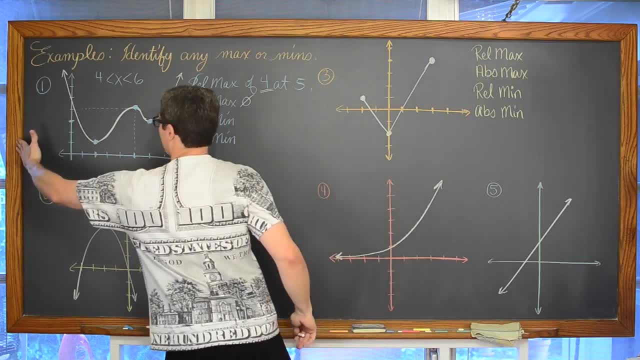 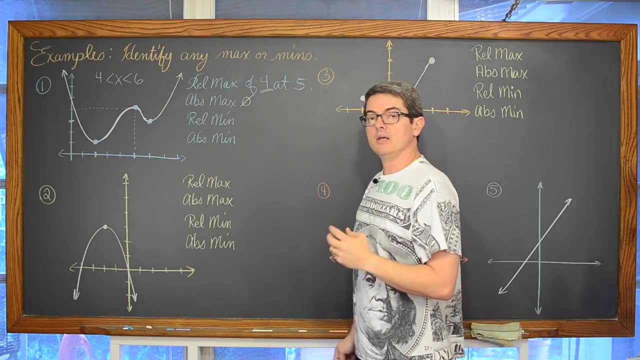 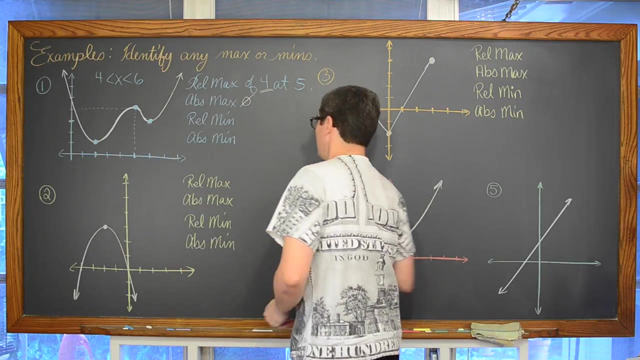 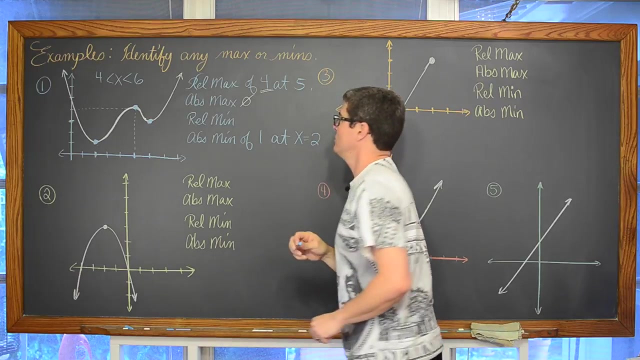 about looking at the entire domain of the graph, You know, including all of the x values from negative infinity up to positive infinity. what is the smallest y value that is included in that graph? or throughout the entire domain, and that is going to be one. So we have an absolute min of one at x equals two, and then 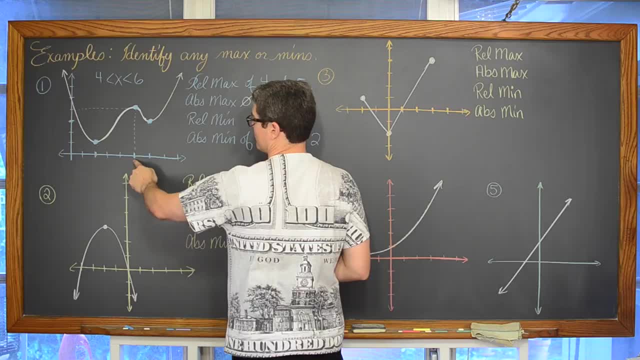 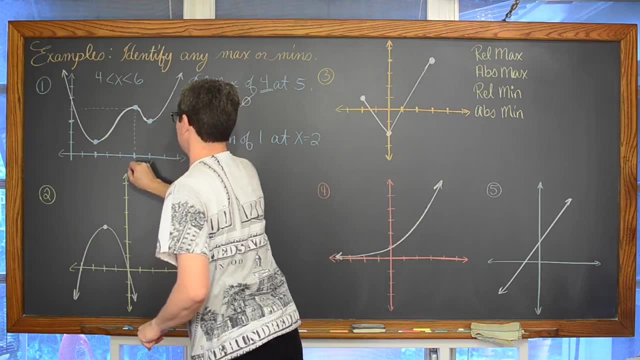 I can see this point here on this open interval. say this open interval from where x equals two. and I can see these points here on this open interval. say this open interval from where x equals two is greater than 1,, 2,, 3,, 4,, 5.. I should have put some numbers on here. I could say really 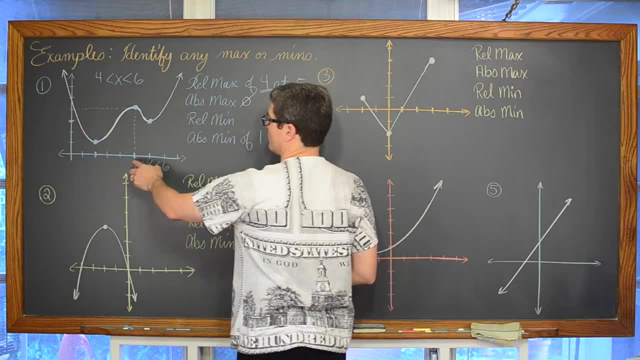 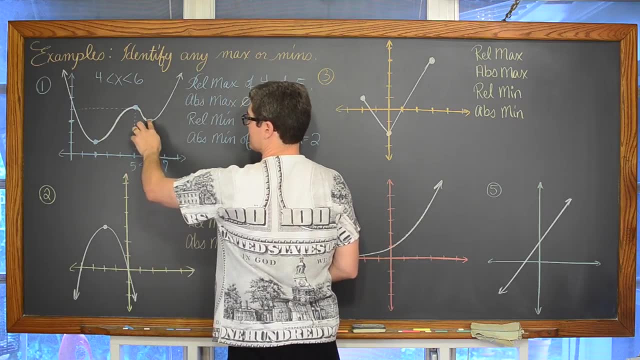 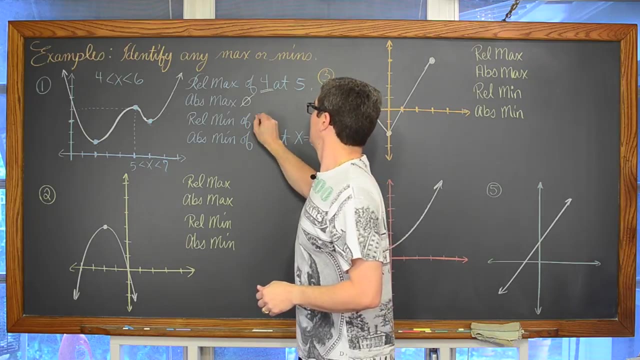 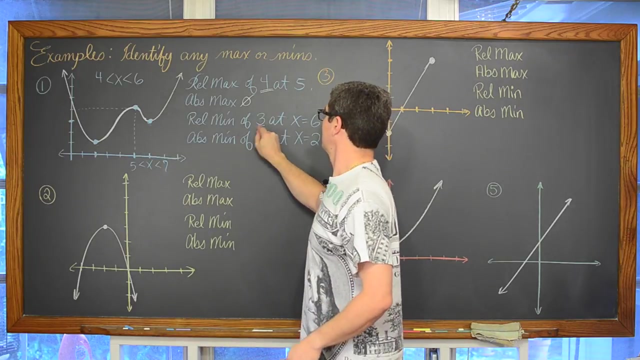 any x value. but let's say x is less than 6. That would be 7, wouldn't it? From that open interval of 5 to 7 the graph falls and starts to rise again. We can just visually see there is a bottom there. That is a relative min of 3 at x equals 6. Again, your book might. 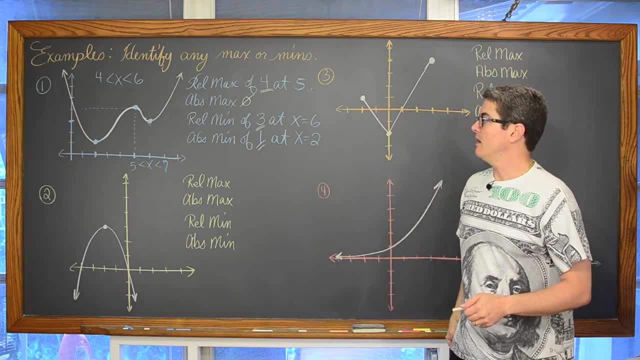 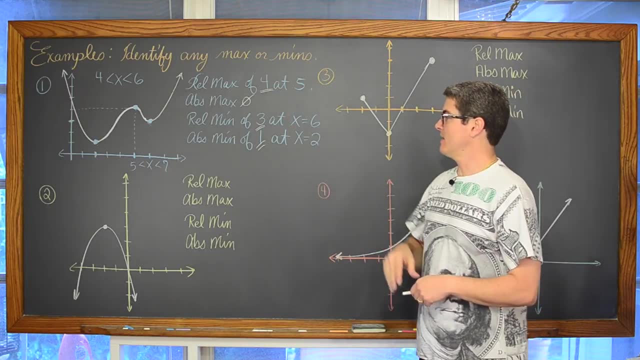 just be using the 4,, the 3, and the 1 for identifying the extreme values, The maximums or minimums, whether they are relative or absolute. For this graph here, I am going to use the x value. I am going to use the x value of. 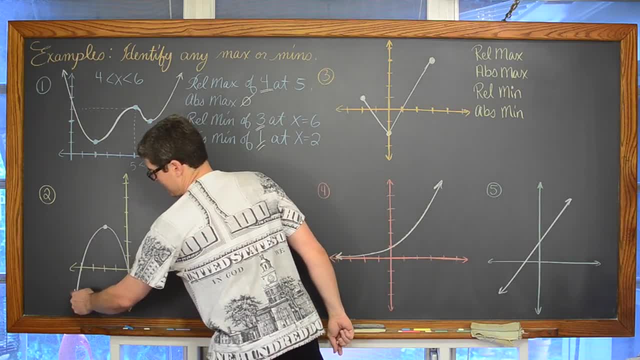 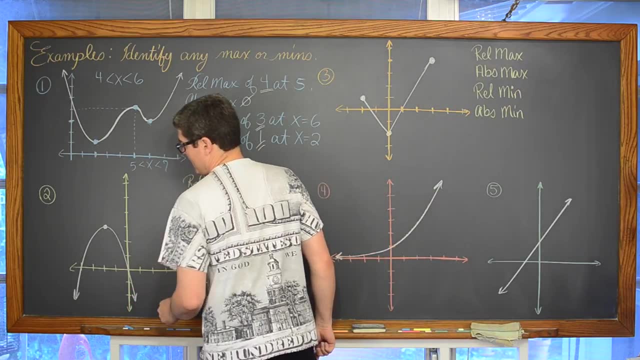 7. We have another graph that has end behavior, which is the same. It is going down to the left and down to the right. It is a parabola. It looks like a parabola anyway. It is opening down and throughout the entire domain. there are no breaks in the graph. It is a continuous. 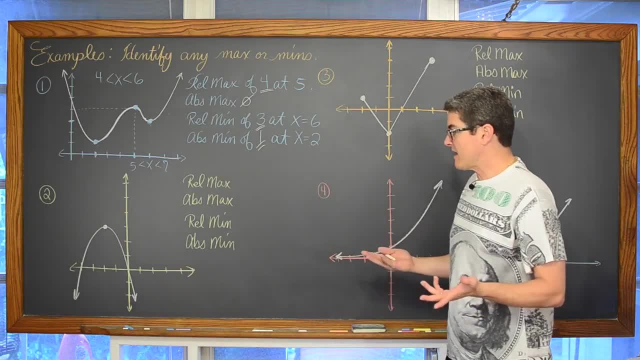 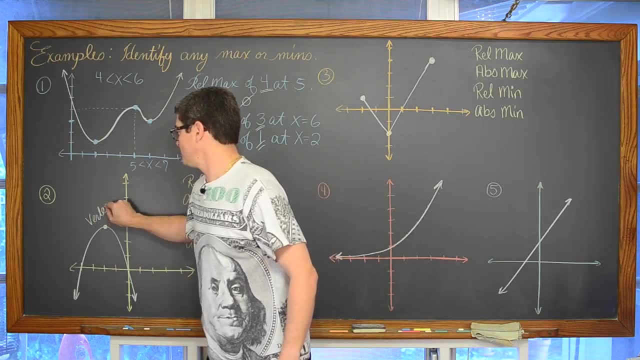 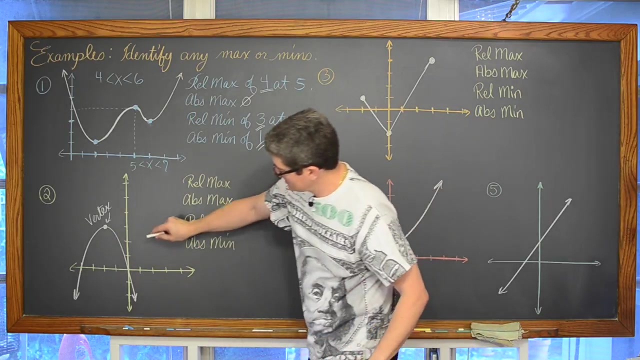 curve going to the left and right forever. I can clearly see that there is a top to that parabola. Later, if you haven't studied parabolas, we will know this as being the vertex We need. the y-value of that vertex appears to be 3.. We have an absolute max. where is my 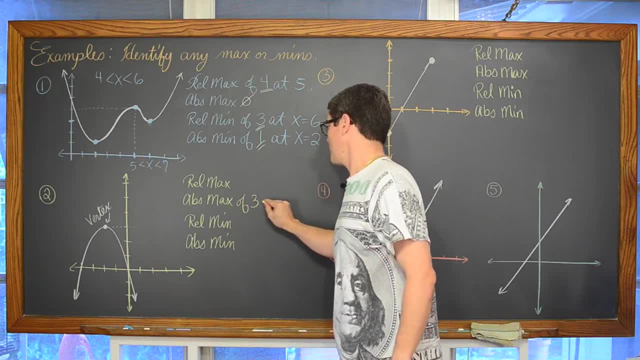 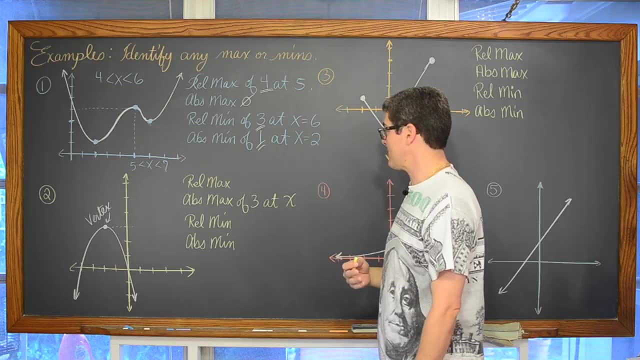 yellow chalk of 3 at x- and I am just writing x to be redundant- if you really understand the language of identifying absolute max and min's- Maybe we don't, because we are learning it. So we have an absolute maximum y-value of 3 at the x-value of negative 2.. We have 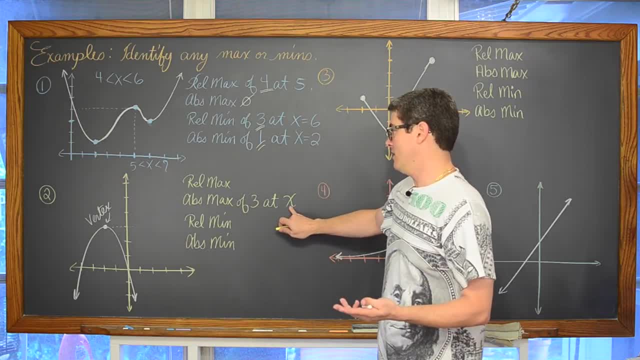 a 1 based equation for the x axis as well, because this tool has some make & make understand about the method for doing that. Let's bring this back to the question here. So if you won't проinga, you won't find that eraser tool here anywhere. I have a point marker there. 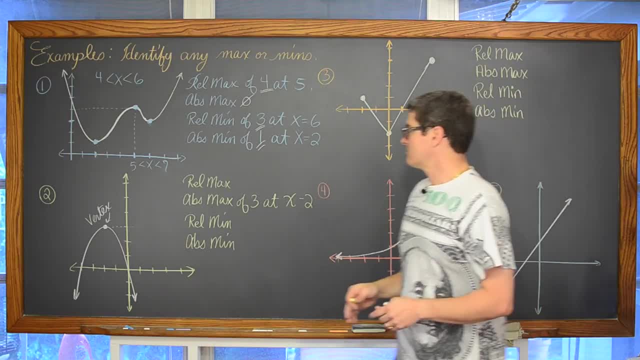 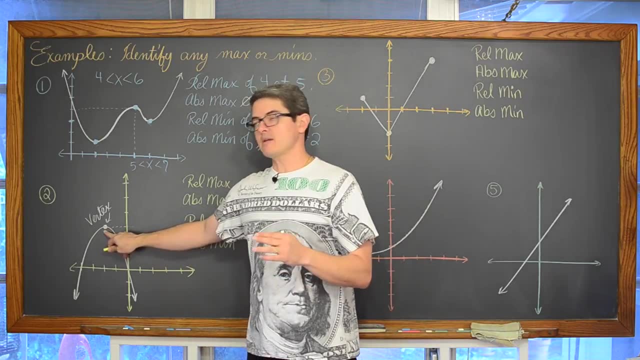 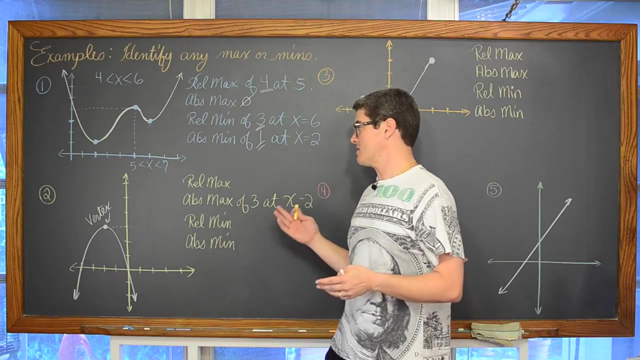 2. Now a relative max. well, there is only one maximum in the graph, so really I guess there is some kind of open interval where that y value of 3 is going to be the largest y value, but it also is the same as the absolute max. So the relative max and the absolute. 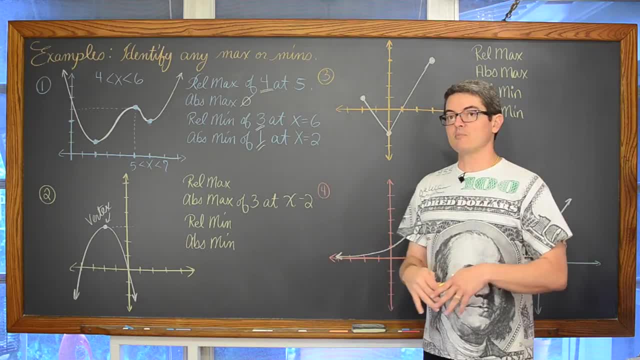 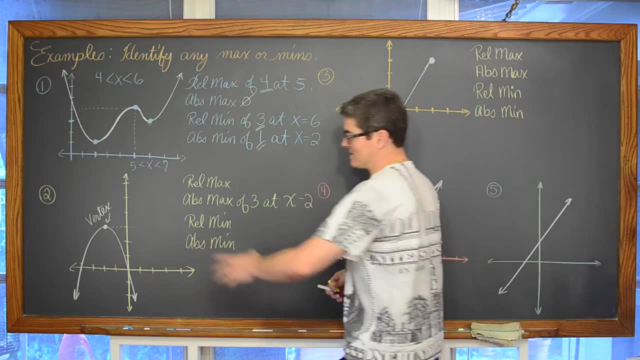 max are kind of the same thing, but the absolute max is more of a special case because it covers the entire domain. So I am just going to identify that as our key point of interest. Now the graph goes down forever. There is no where. as you read that left to right, that it kind 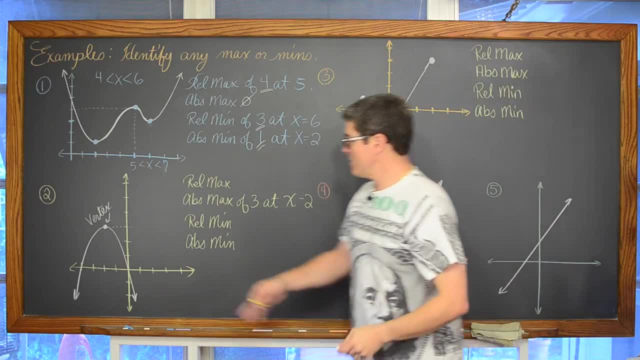 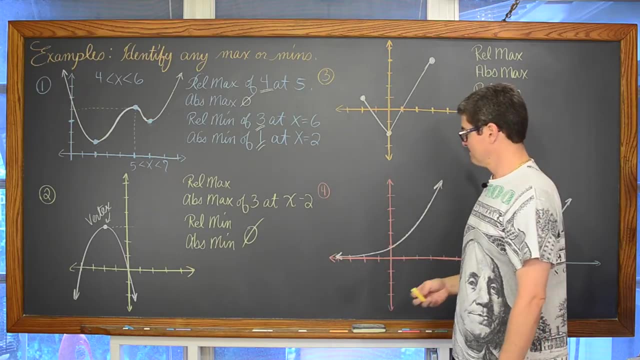 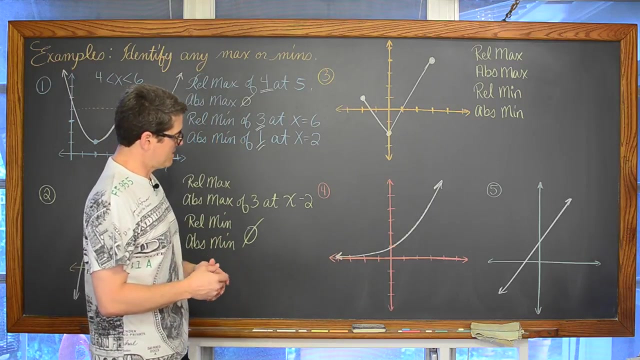 of falls and rises back up again. So there is no, because it goes down forever. there are no relative mins, or absolute mins, for that matter. Now, over here we are going to play with this third example a little bit. It is a great example and I also find it a 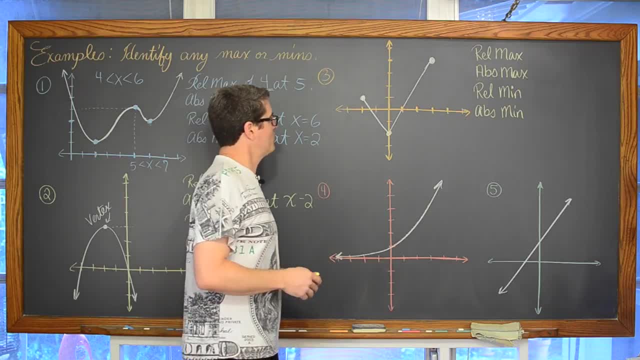 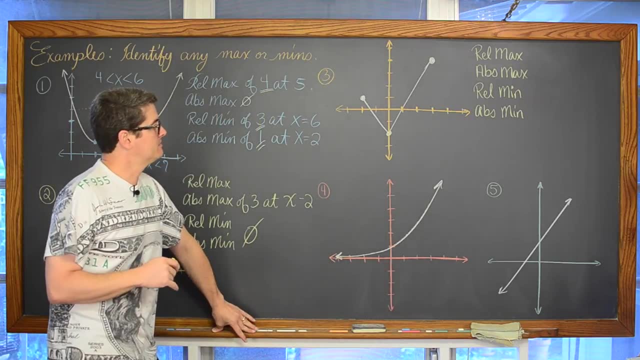 tad bit frustrating. We can see. let's see here. is there a relative max? I am going maximum value. That is the one that I kind of struggle with: the way that relative maximum is identified or not identified, but defined. I checked three textbooks just to make sure. 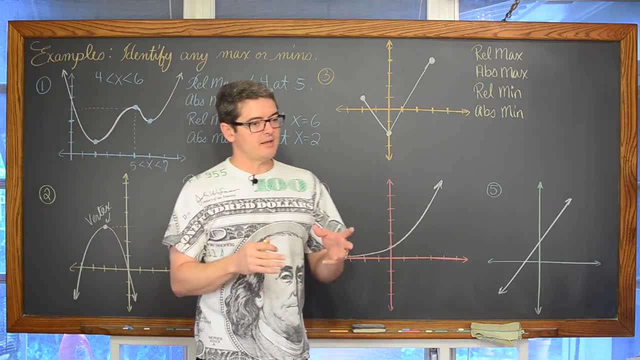 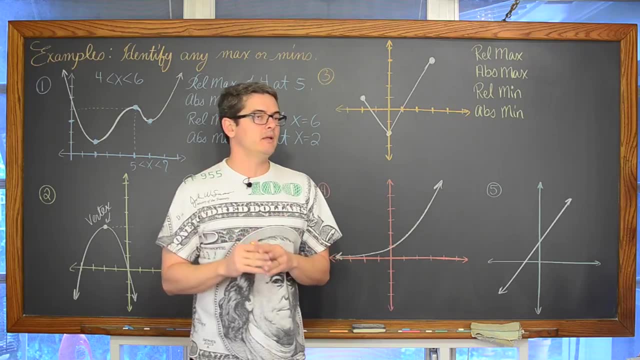 I was going to say it right in this lesson. A relative max was about that a within an open interval, such that f of a was greater than f of x on an open interval. I can see that there is sort of like a top value here. This is at the point. negative two left two. 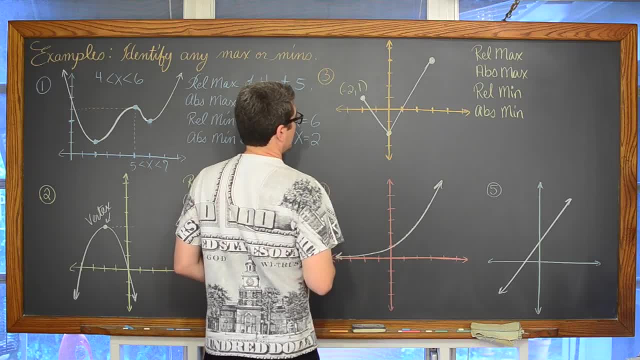 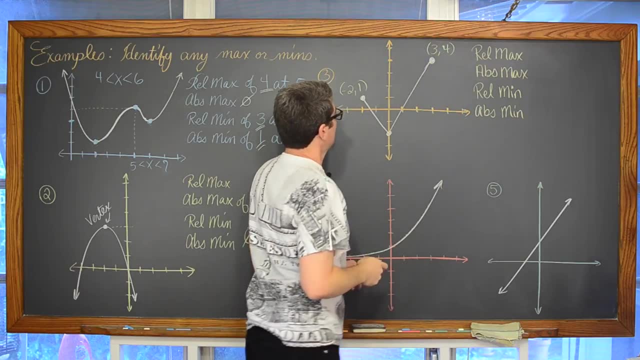 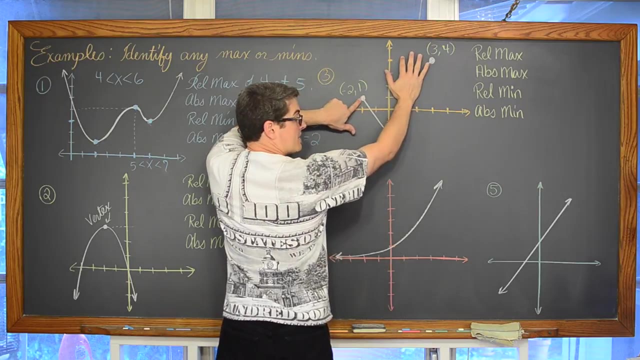 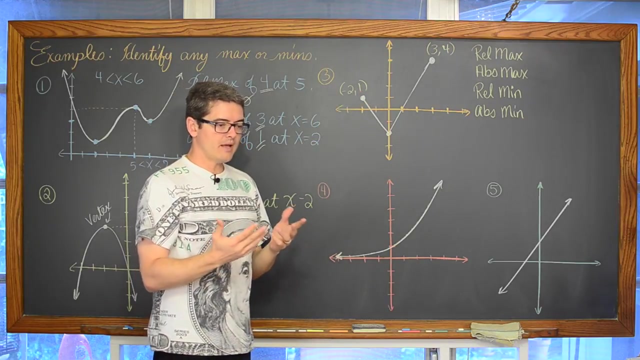 and up one. So this is the point. negative two: one. Then we have a point over here of three, four. Well, if I just look at this portion of the graph, then that seems to be some kind of maximum, But I can't identify the one at negative two as a type of maximum which really 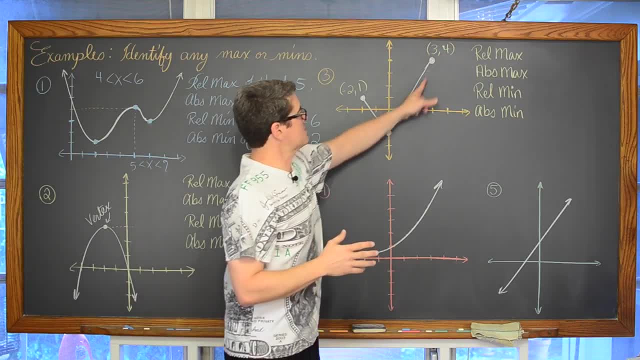 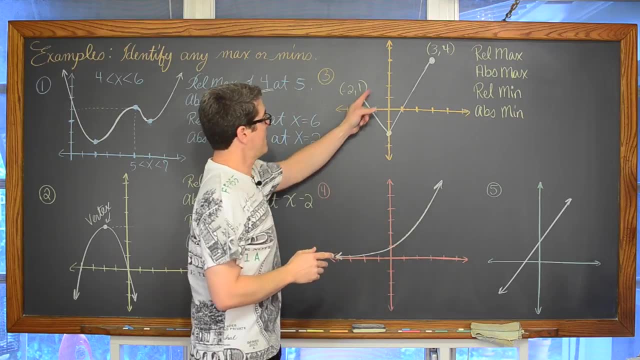 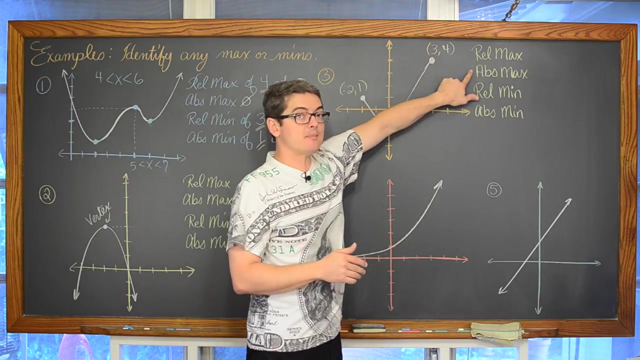 seems weird Because over this, This entire graph, I know there are not arrows extending on This, is it? It starts here, falls and goes up and stops. There are no arrows. There is a maximum of four, at three Within this entire graph. that four is an absolute max. That value of four is greater than every. 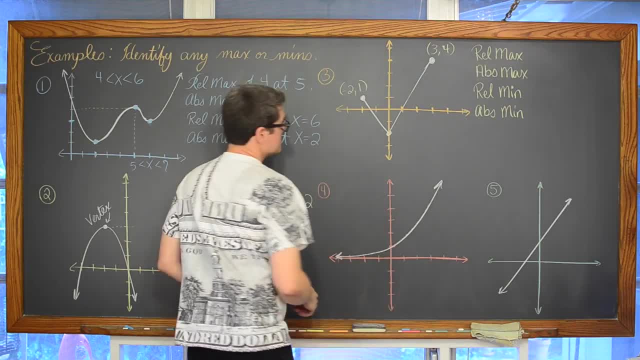 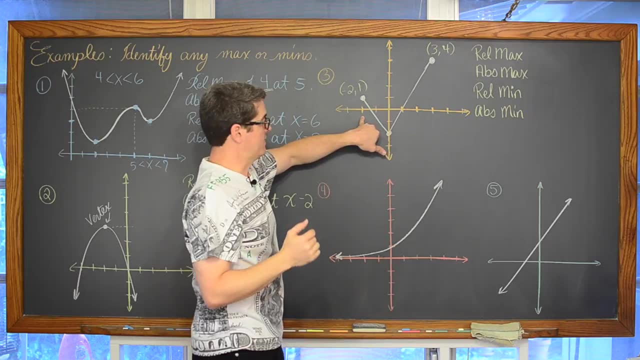 other y value within this function's domain. By the way, the domain of this function is from negative two to positive three, including those values, The range. I have another lesson about identifying domain and range from a graph, which I will put a link here. 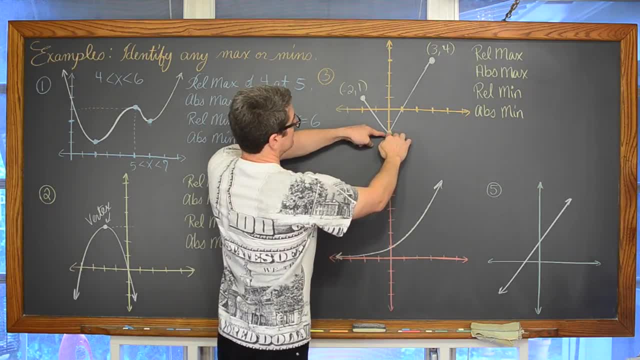 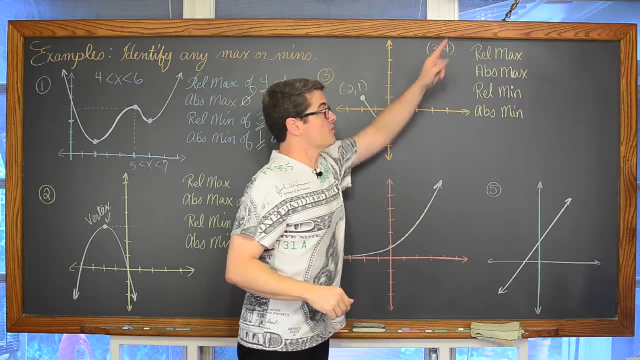 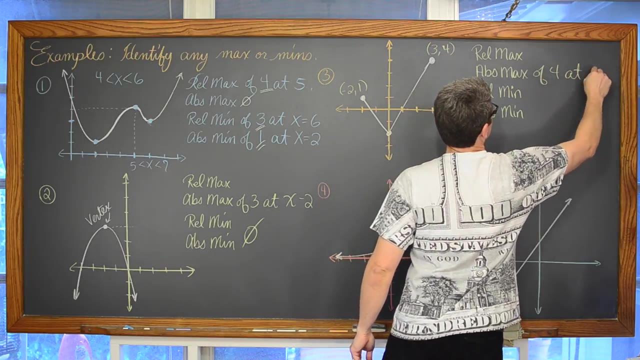 if you need help with that. The range goes from negative two up to positive four. Within that domain of negative two to positive three, four is the biggest y value, So we have an absolute max of four at x equals three. Again, that four is the maximum value that we are. 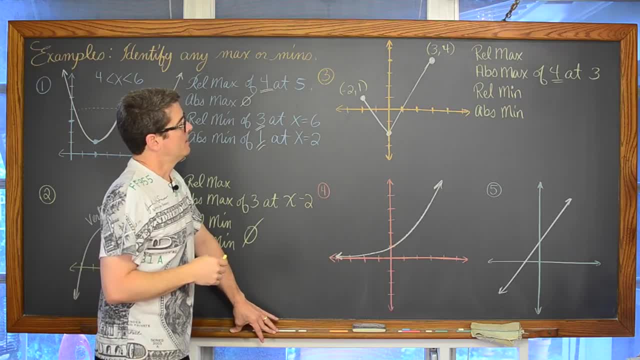 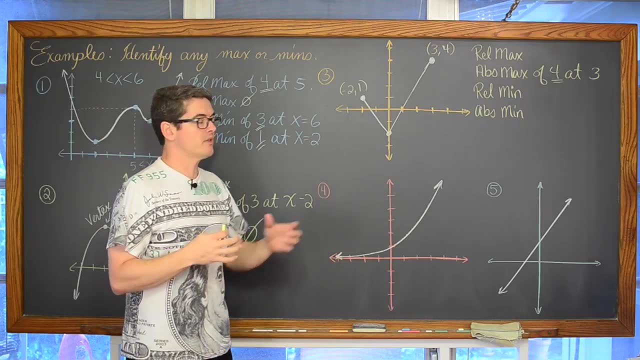 concerned with. I am just adding in a little extra information. I really want to say that we have a relative max of one, at negative two, but I have checked three textbooks and none of them would identify that point as anything special. It is just. 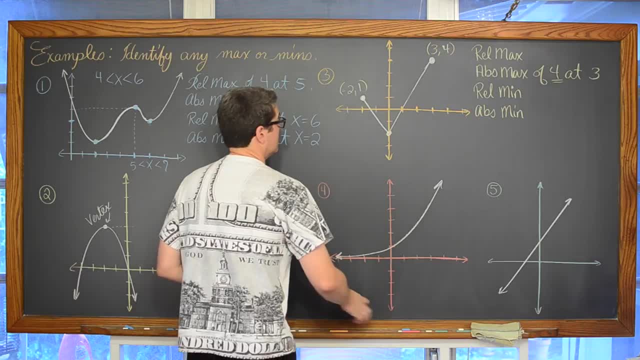 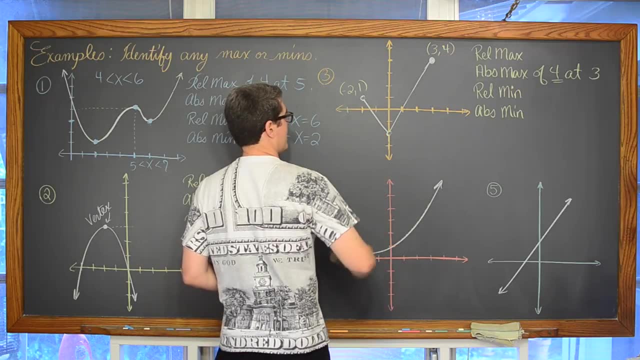 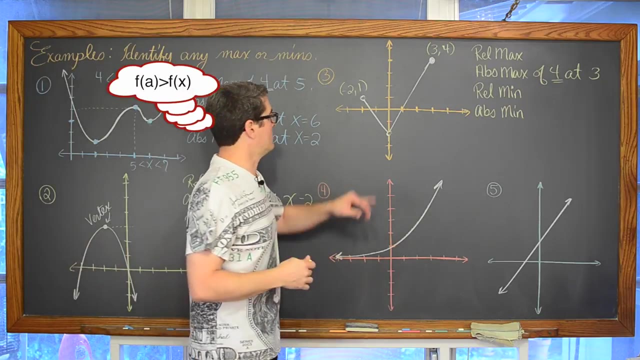 an end point, Because when you are identifying a relative max, all the definitions say that when you are identifying a relative max, it needs to be on an open interval, That there is an a on an open interval, such that f of a is less than f of x. Well, if you are going, 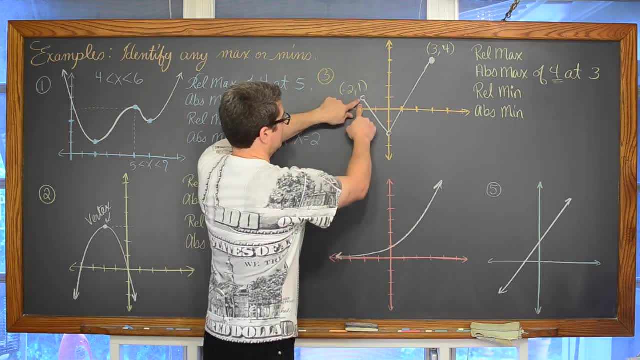 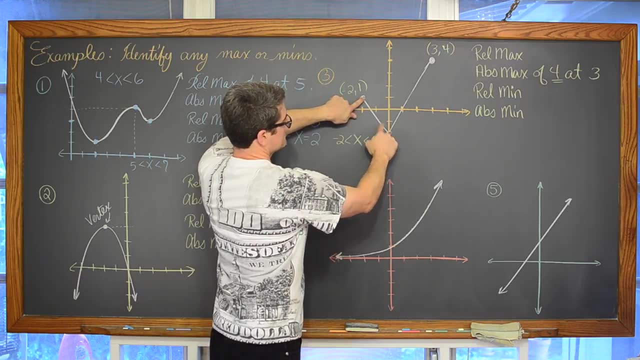 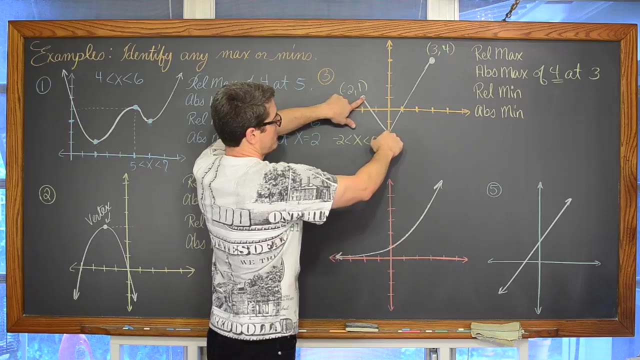 to do that. if I make those dots hollow, indicating an open interval from negative two to zero, then there is no place where the graph goes from falling to rising- Well, we are talking about maximums. There is no place where the graph rises and then falls again That negative. 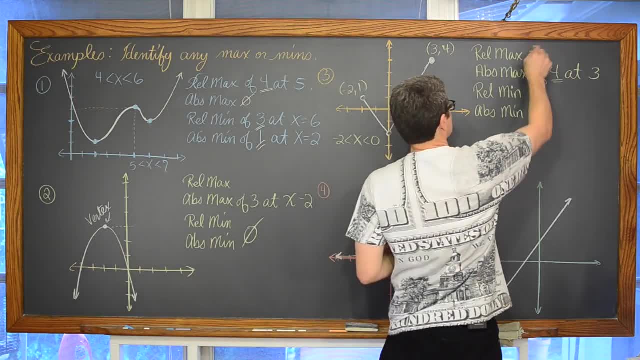 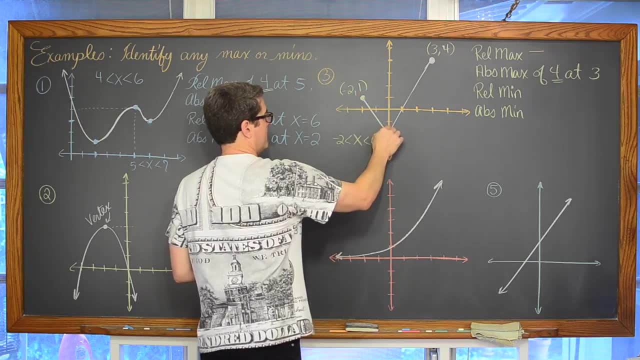 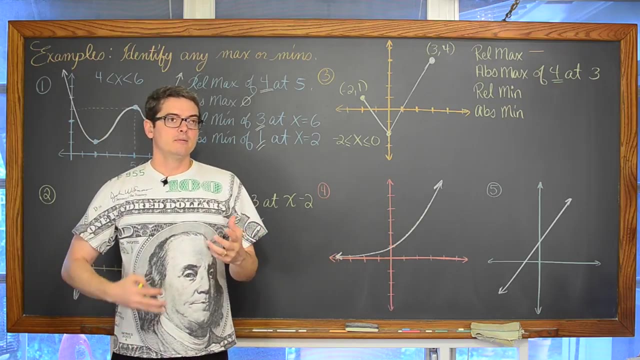 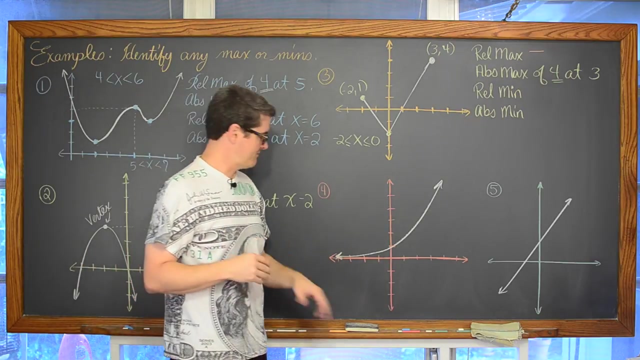 two. one is just an end point, So no relative max would be identified because that would be at the end point of a Closed interval, And identifying relative max and mins are always about identifying a lowest y value, if you will, on an open interval. So sorry, I just find that a little. 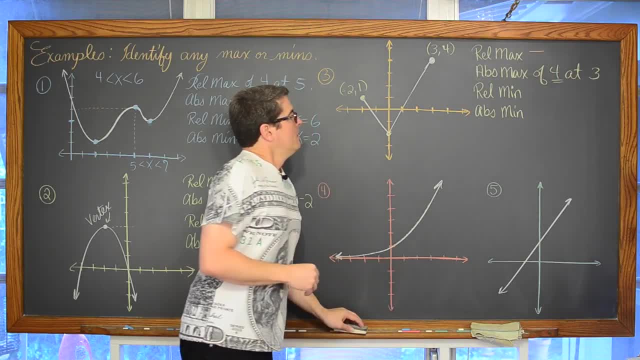 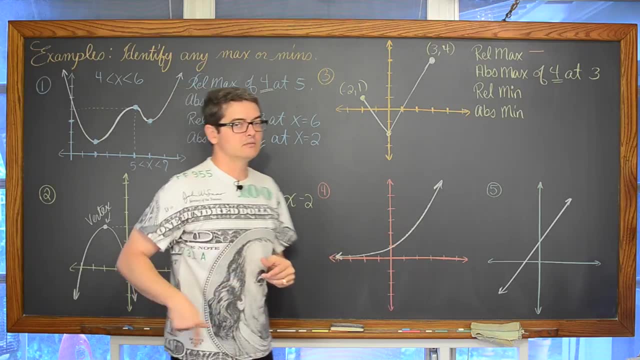 bit bothersome, But that is the way it is. So, relative min. well, there is only one point. Oh, I hear the static. Let me try changing the channel on our radio here. Ok, let's see if that helps. 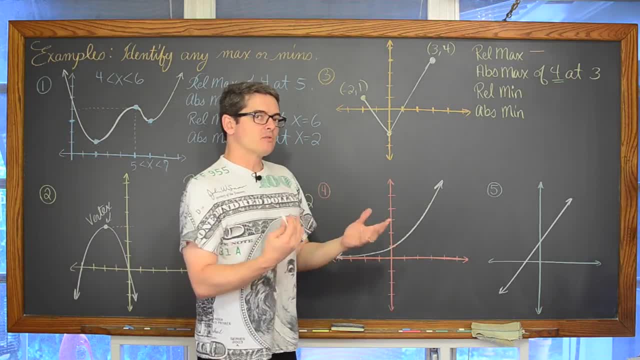 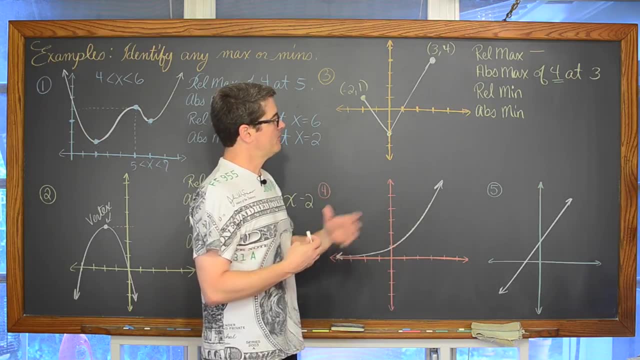 So we only have that one minimum value. So the relative min and the absolute min are kind of they are going to be the same point, if you will. And again, that absolute min is: well, I am just going to identify it there We have an absolute min of negative. 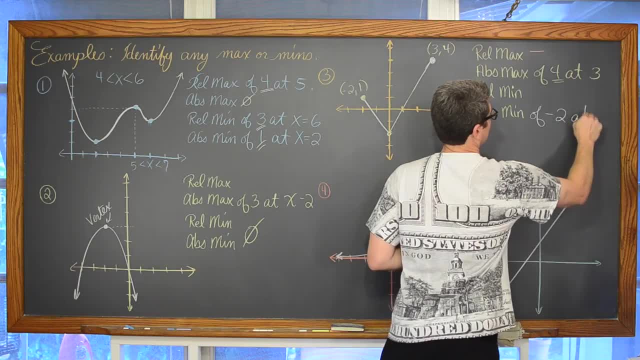 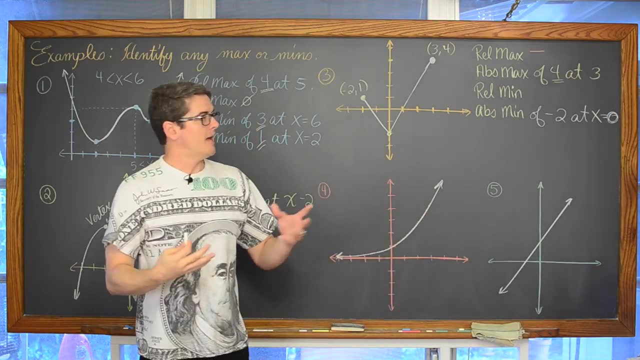 two at. in this one I will write the x at: x equals zero And the relative min, absolute min, kind of the same thing, or at least are the same point. The lowest y value in that entire domain is negative two. So we are going to identify that absolute min of negative. 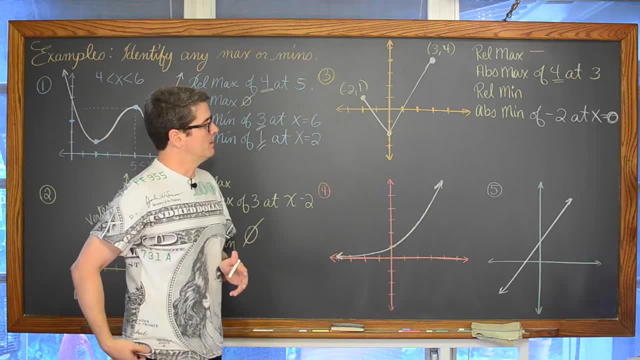 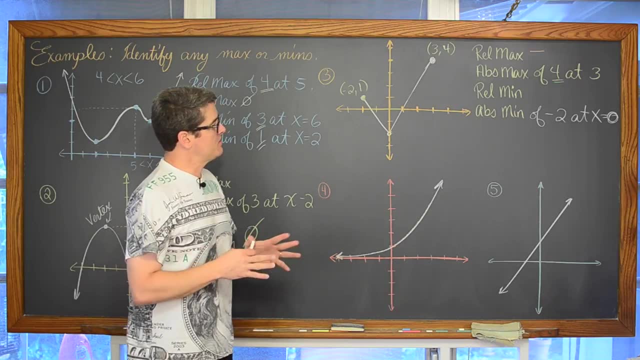 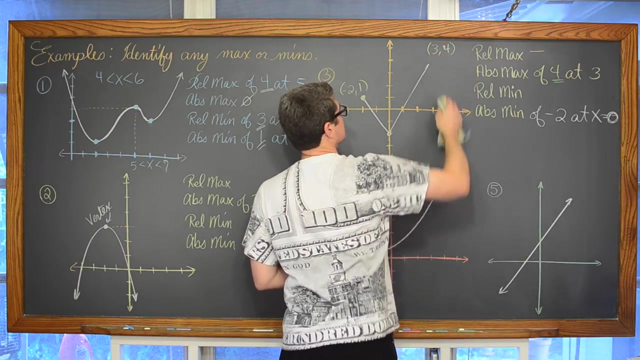 two at. in this one I will write: the x at x equals zero And the relative min- absolute min- at x is equal to zero. Ok, Now let me change this problem up a little bit. If I were to make this dot open, then there is still an absolute minimum of negative two. 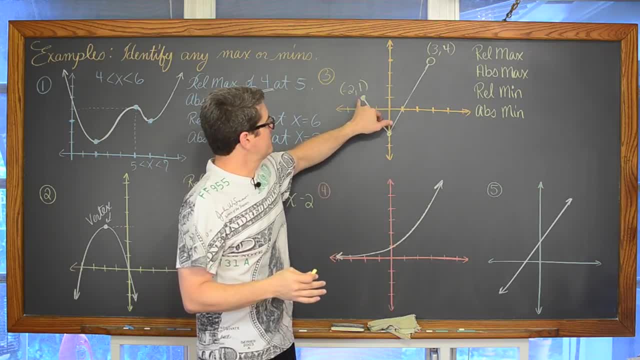 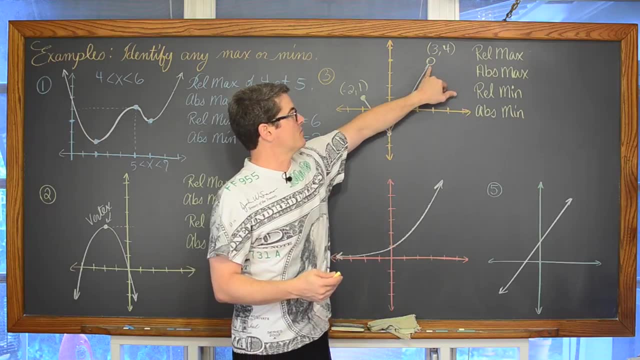 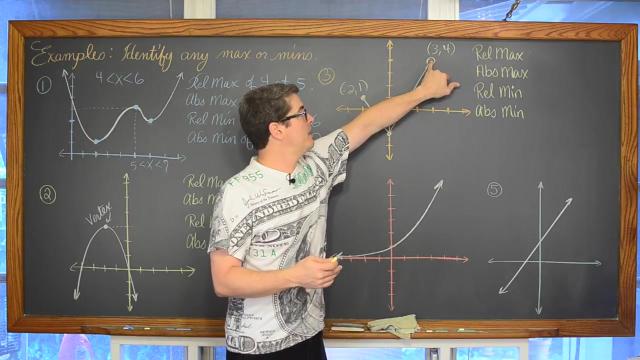 at zero, But- and this has sort of like- it goes to a maximum of one, but then there are places in the domain where the graph goes higher than one. But if that is an open dot, where are we stopping at? Now we are approaching the point .34,, but it is. we are not getting. 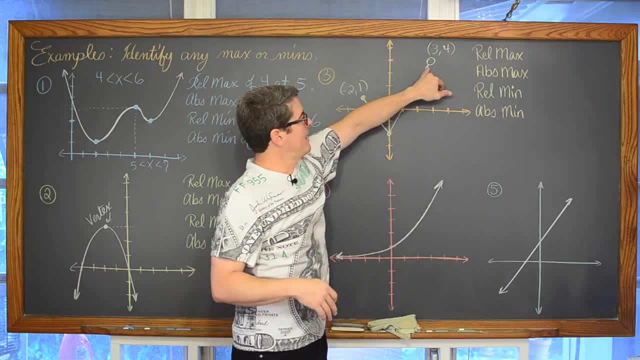 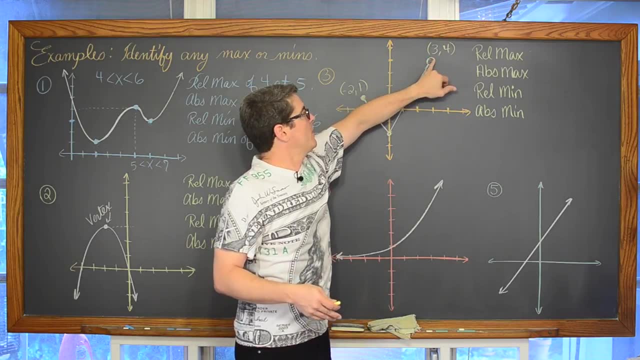 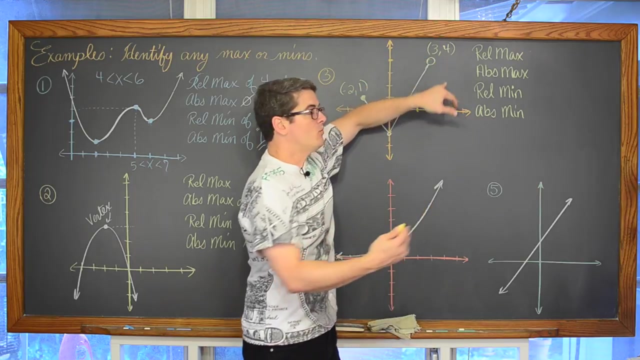 to .34.. We are getting to like- oh I don't know How- about 2.8,, 3.7, or 2.9,, 3.9, or 2.999,, 3.999, or 2.99999999.. I can get infinitely close to that open dot and I am almost getting. 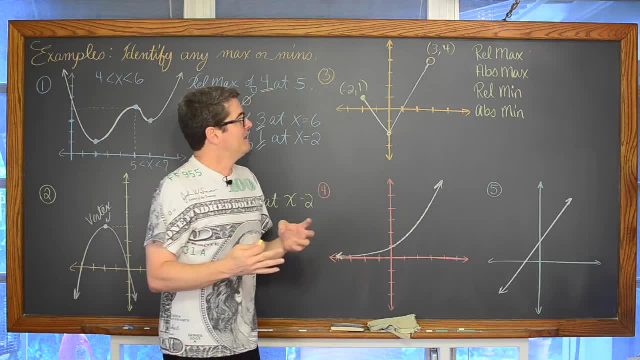 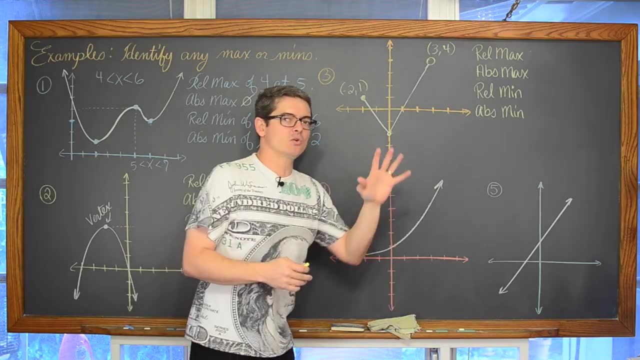 close to wanting to start talking about calculus, but we are only in algebra one. But we can get infinitely close. We can approach that open zero, that open dot- excuse me, but never actually get to it. So I can't say that there is a relative max or an absolute minimum. 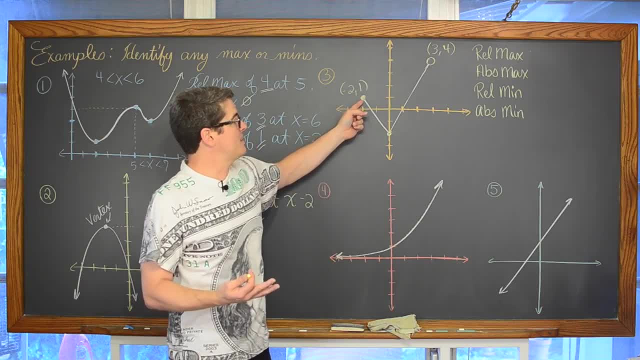 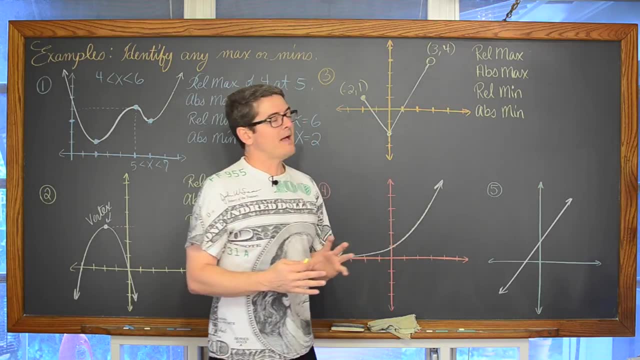 absolute max now, because I can't identify that as a relative max, because it's not going to be. it's on an end point, It's not part of an open interval. Seems really weird to say: And there's not an absolute max because we're getting really really close to that. 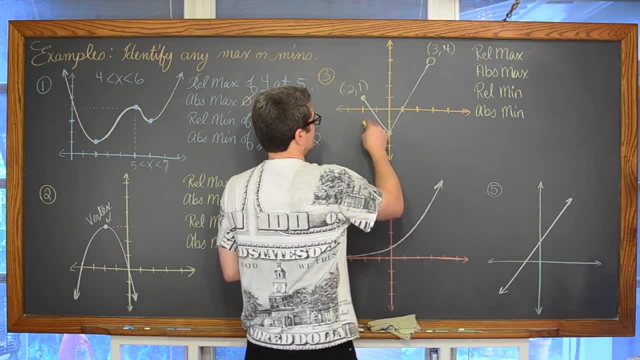 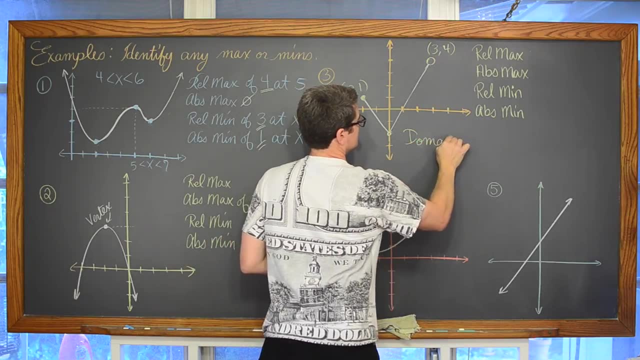 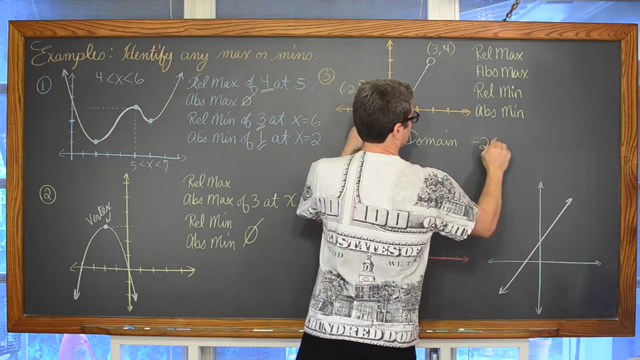 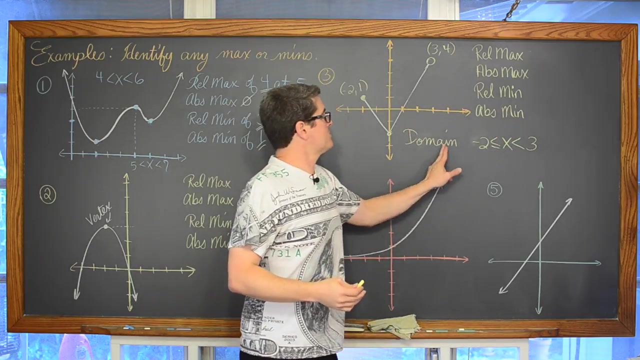 open dot but I'm not including. you know, like if I were to talk about the domain of this graph right now, the domain is all x's from negative 2 up 2, but not including 3.. So if 3 is not part of the domain, then I never get to the point of 3, 4.. So there are no. 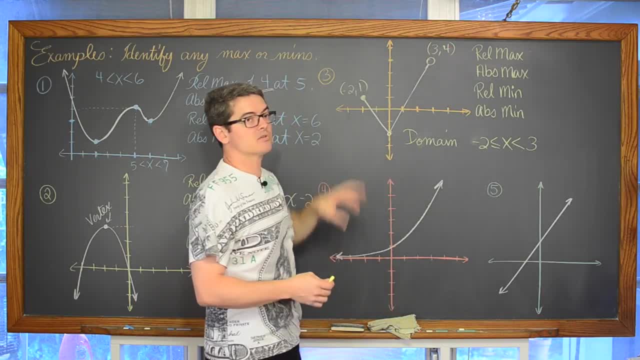 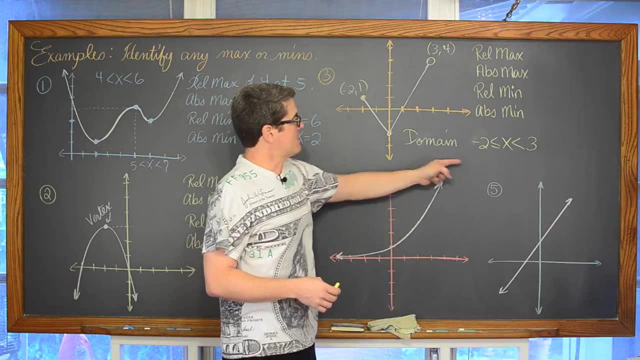 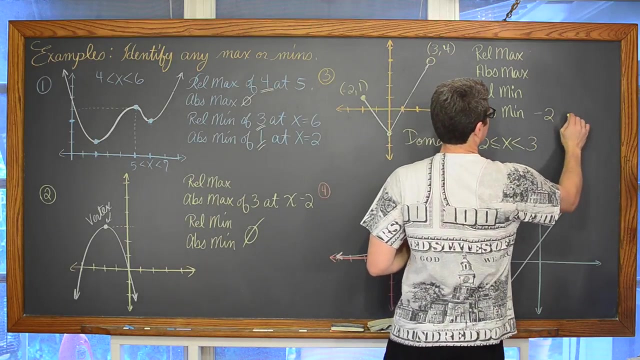 maximums, relative max or absolute max in this graph? Uh Again, can't call that a relative max because it's not on an open interval, We're not identifying it. on an open interval, There's just an absolute min of negative 2 at x equals 0.. Now, if I 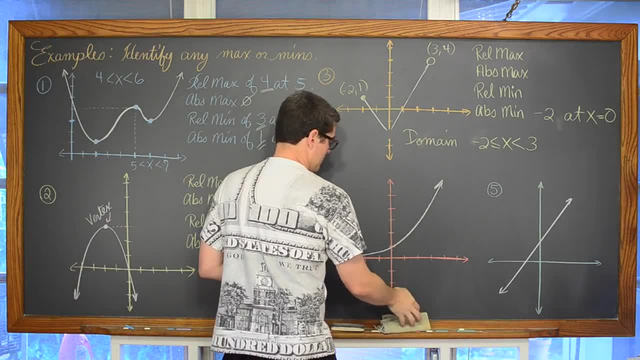 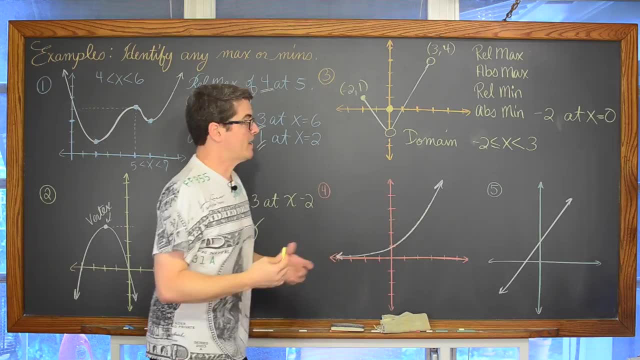 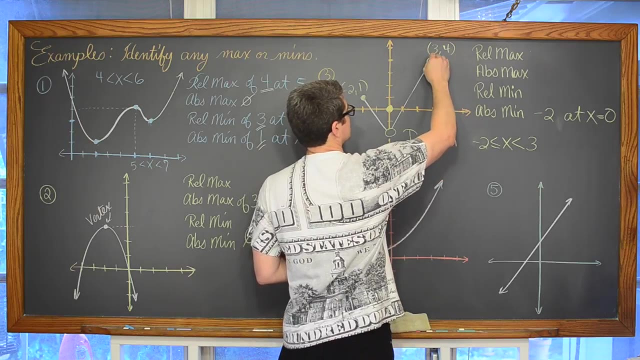 come up here and I just mess with this a little bit more and I make that an open dot and then maybe I put a dot right there. so now the domain, Let's leave that open. Now, if I just again put an open dot where there was one at the 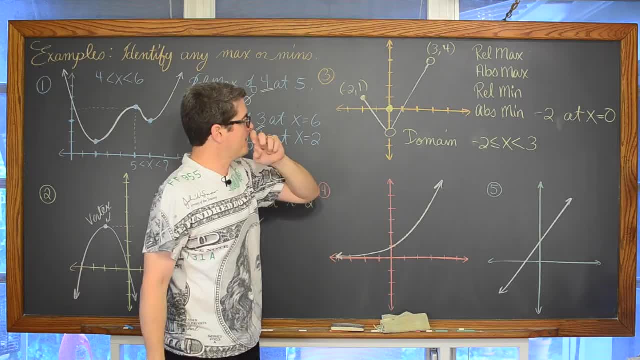 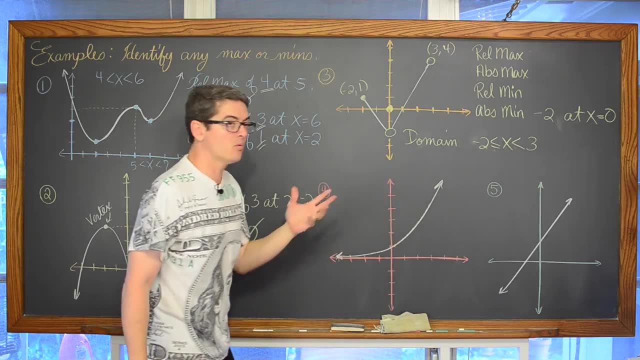 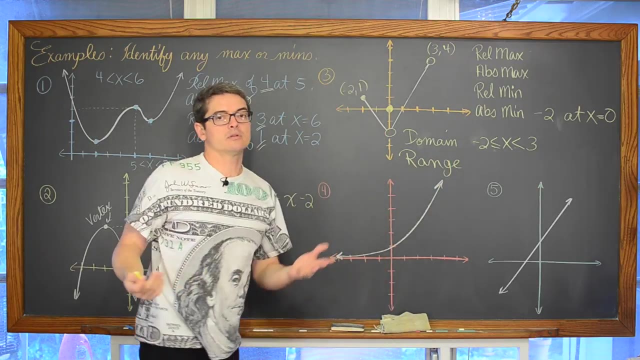 sharp bend and put it up here and then pop it up there. my domain is still going to be from negative 2 to 3, with an equal sign and an open inequality. The range: What y values are included in this graph, At least the way it's drawn right now? Do we have a y value of negative 2 or does it? 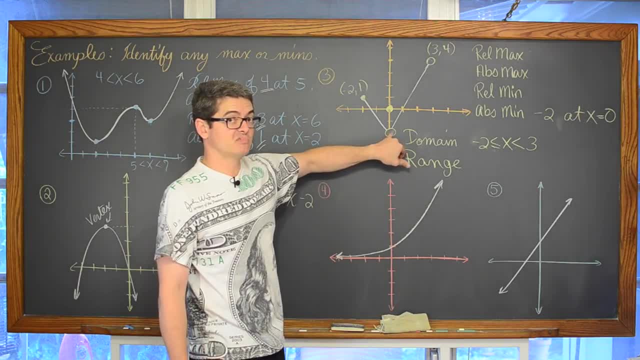 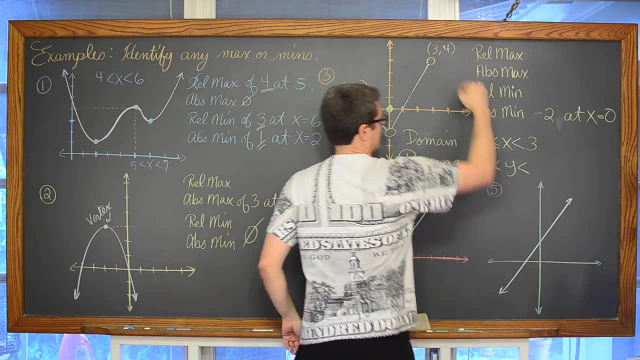 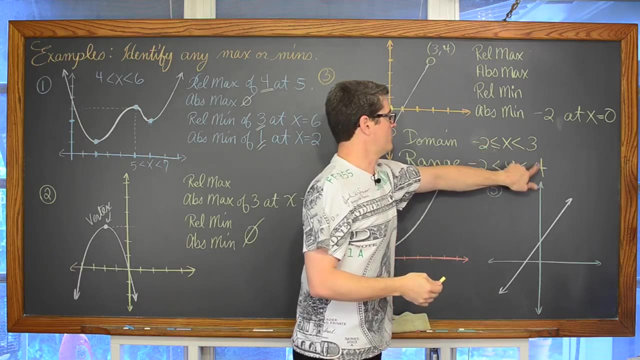 just approach a y value of negative 2?? It's an open dot, So our y values are going to be greater than negative 2 and less than, again, not actually reaching that point- of 3, 4. but we're approaching that open dot of 3, 4, which means that x value of 3 and 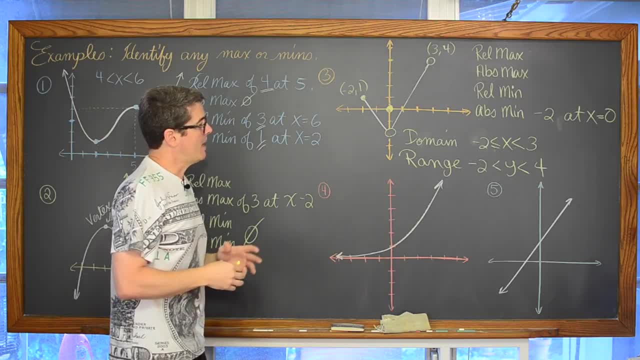 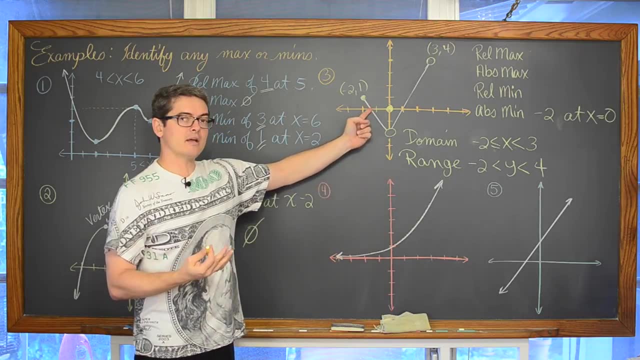 that y value of 4 really can't be included in the domain. Now is there an absolute min. Is there a graph at y equals 0? Right there and there. Is there a graph at y equals negative 1? Right there, and there. Is there a graph at y equals. 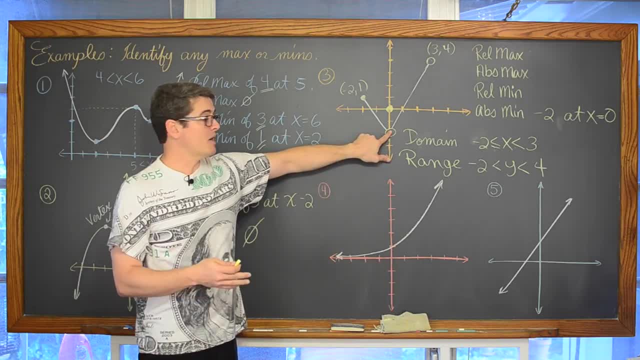 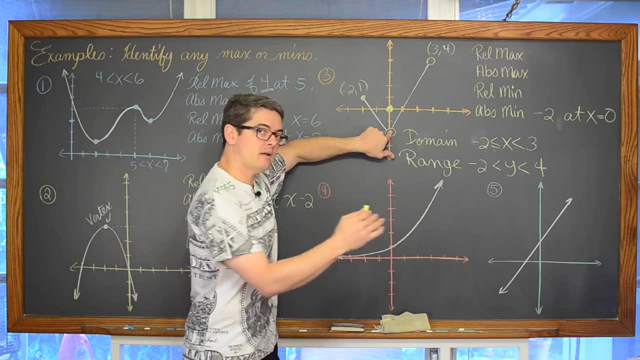 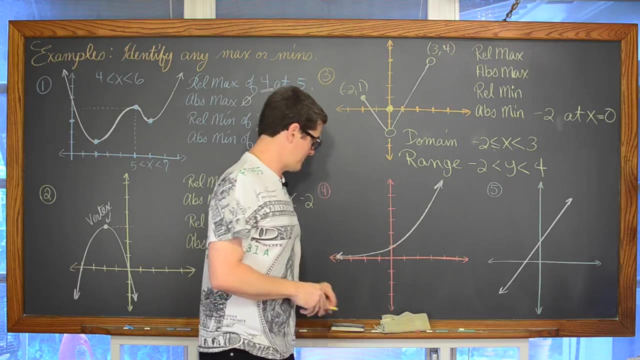 negative 2?? Not if there's an open dot. It's there. Is there a graph? at negative 1.99999999999999999999999999999999999999999999, Yes, but not at negative 5. too, And the way this graph is drawn: there is not an absolute min or relative min There. 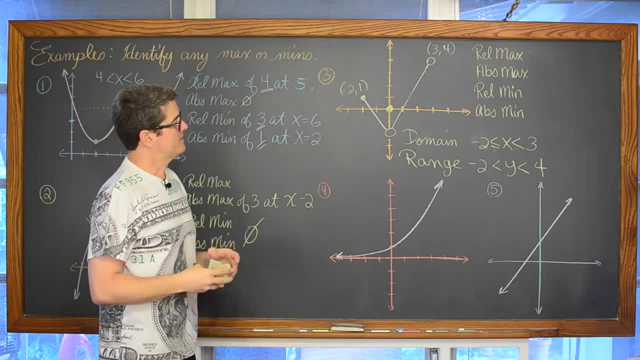 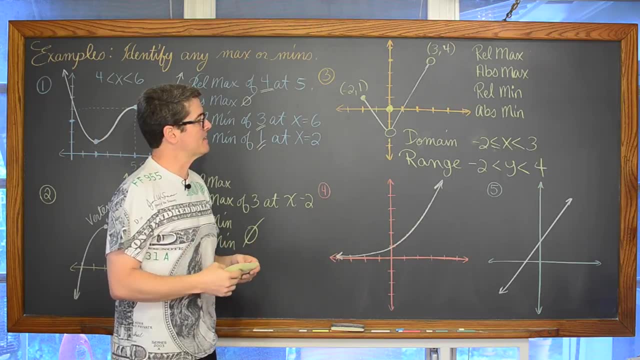 is not an absolute max or an absolute max, And so they can get a little bit tricky, these problems of even just looking at a picture of identifying relative and absolute min and maxes. Oh, let's see here. How about just one more variation, If I come through here? 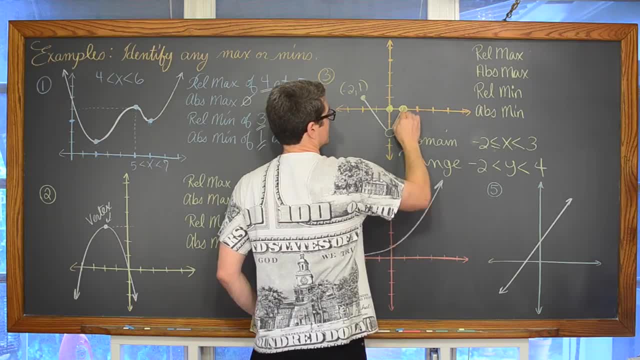 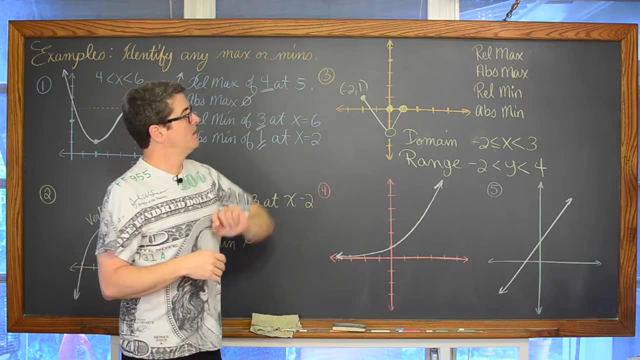 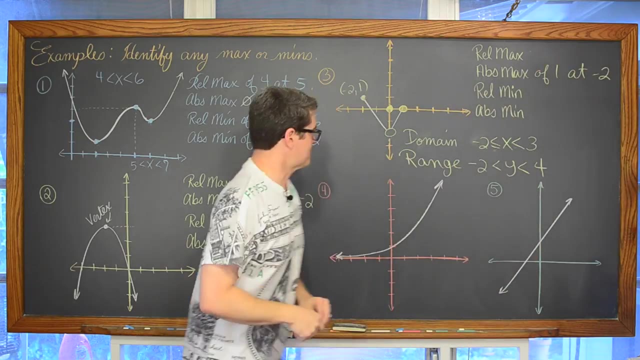 and let's just put in: it doesn't really matter an open or closed dot there. now that point would work for at least the way it is drawn now. an absolute max of 1 at negative 2.. Ok, I don't know how many examples that was, I just did, but it was all off of that. 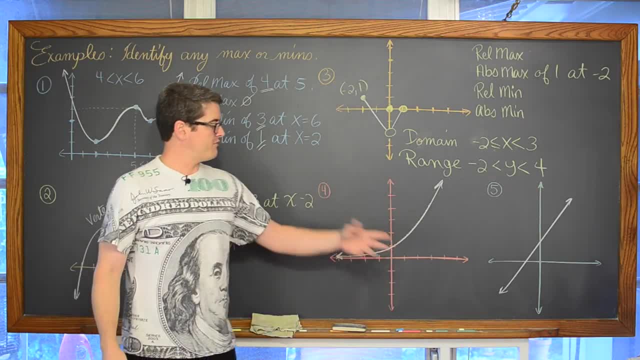 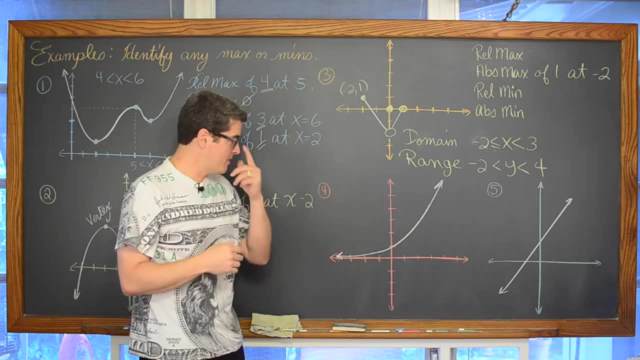 picture. Now, these last two problems, these last two graphs of 4 and 5 have kind of scrunched them down into the corner. Why is that? Well, it wasn't quite because I was running out of room, but it is also because I was running out of room. It is also because I was running. 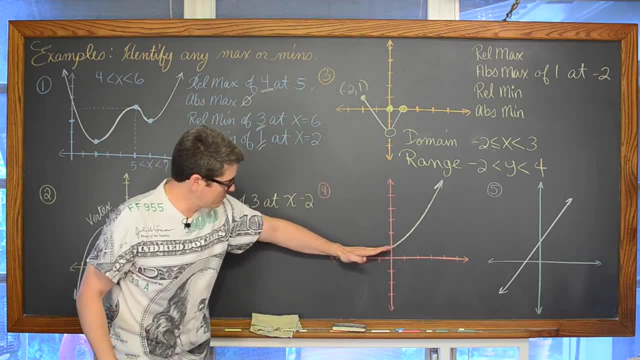 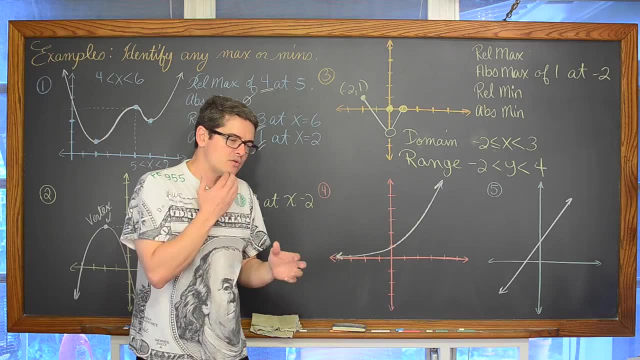 out of room, but it is also because I was running out of room, but it is also because this graph goes down as we go to the left. That graph is going down forever. Now it seems to be flattening out, but do you know something called an asymptote? We are very early into. 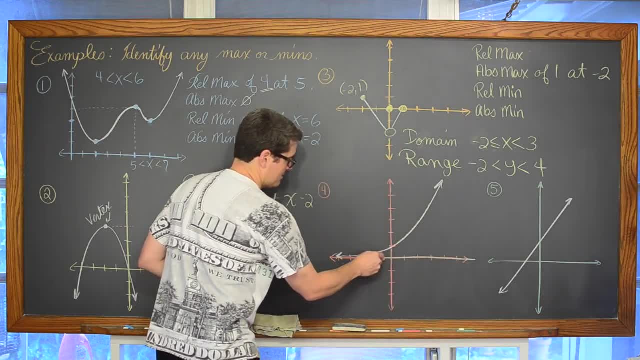 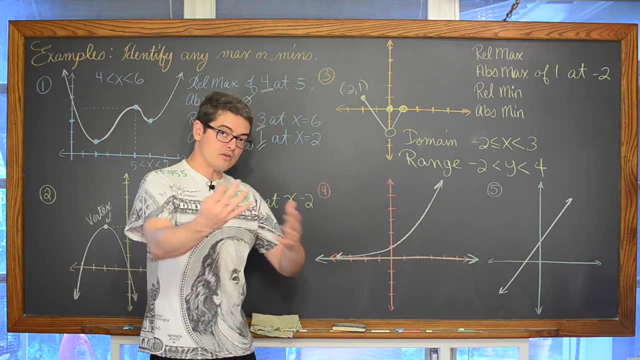 our study of algebra. at least that is how I am making this lesson, and I don't think my book has identified what an asymptote is yet, So that can be kind of a problem. I have to clear that up with my students. I am not sure if you have heard about asymptotes yet either. I will put a link. 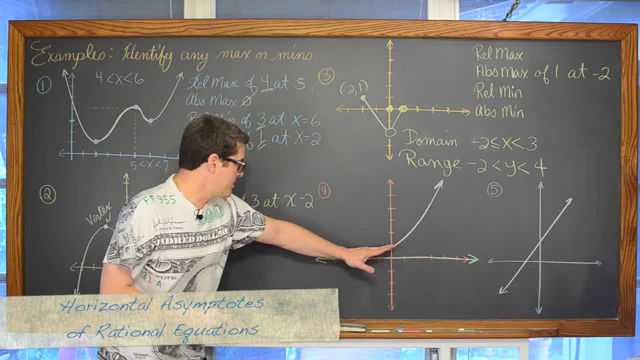 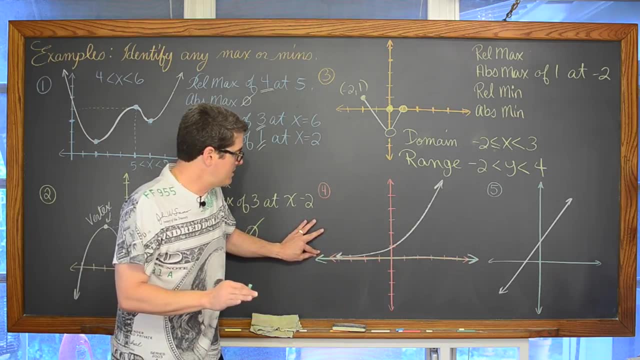 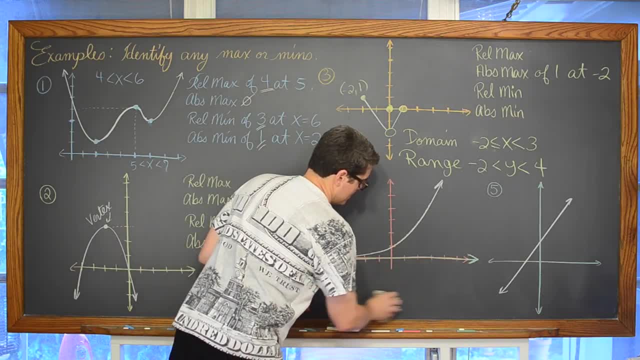 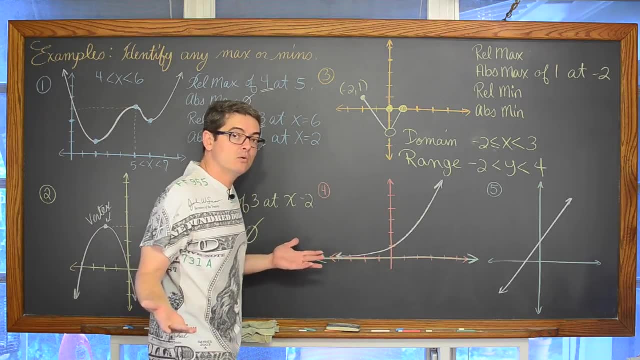 I really didn't intend on making a lesson about domain and range. I have already done that. but understanding how to set up domain and range will explain why this graph has no maximum or minimums- Fancy name for it, but it is a little bit more complicated than. 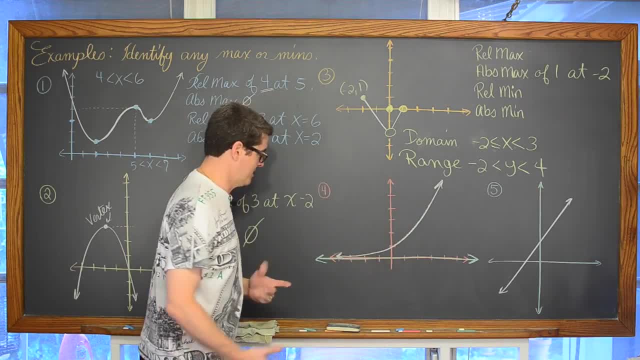 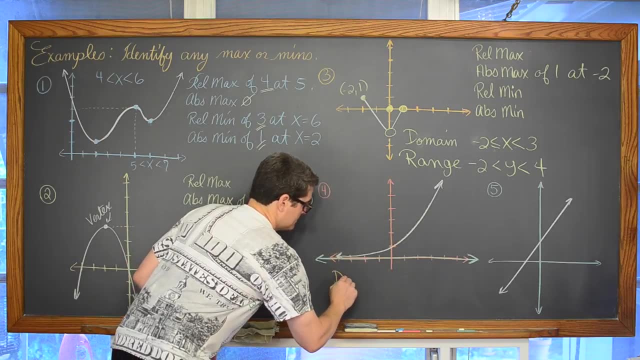 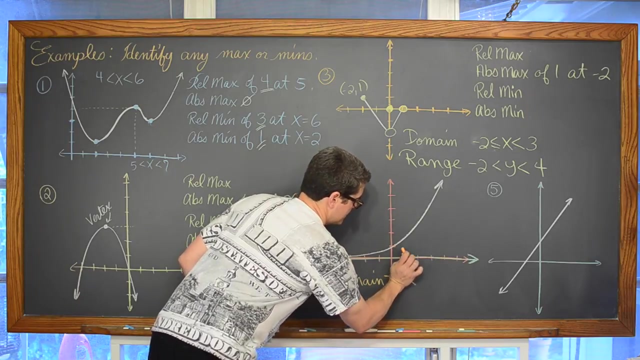 you might think As you read it: left to right, it is always going up, It is monotonic, increasing. That is something I have defined for my students already. The domain of this graph goes left and right forever. So the domain is: x is greater than or equal to negative infinity, not negative. 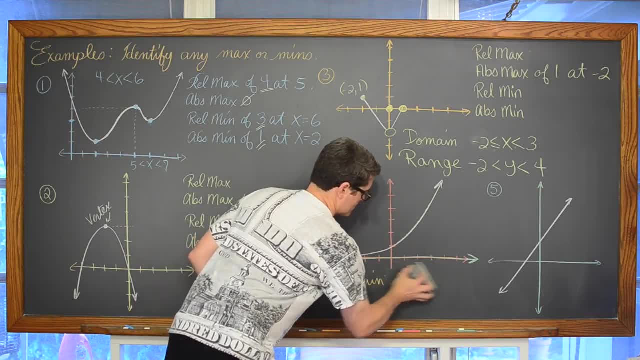 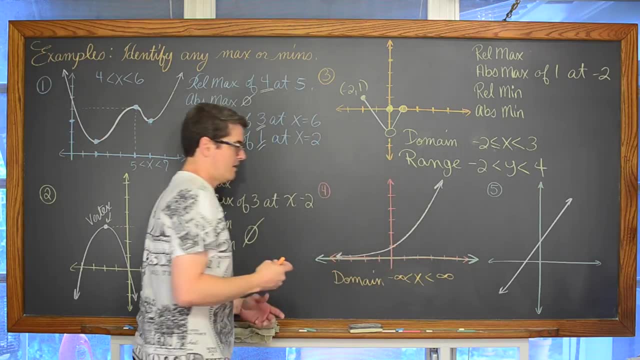 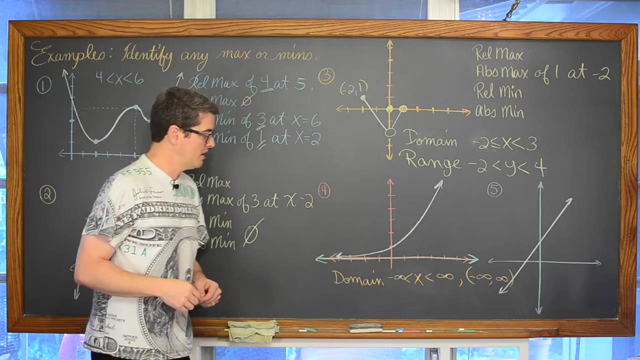 eight. Whoops, I can't write it that way because it is sort of a theoretical number. X is greater than or equal to negative infinity and less than or equal to positive infinity. You might see that as negative infinity to positive infinity if your book is using interval notation. 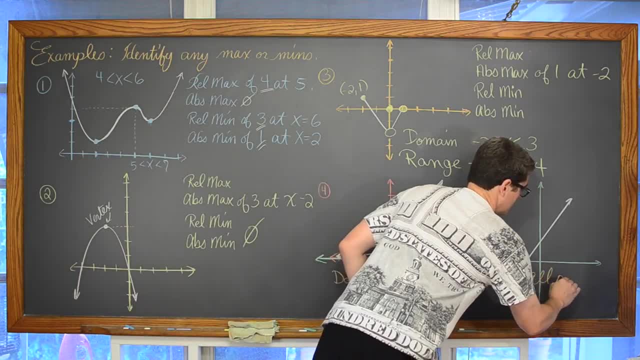 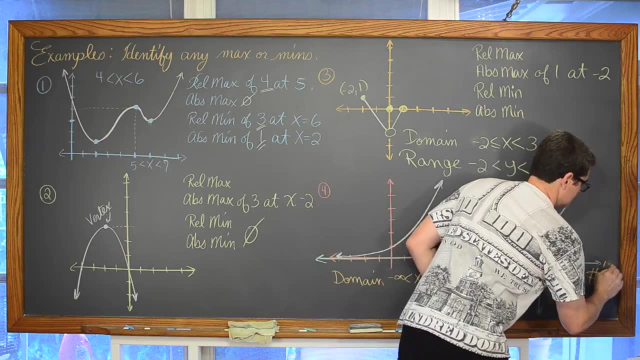 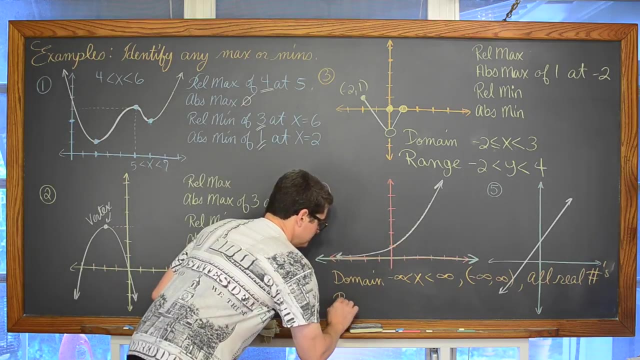 Your teacher might also just say that this domain is all real numbers, Just to put it in sort of English, not number 15.. Well, it still looks like 15, there we go Now. the range, the output values, the y values, if you will, are going to be less than or equal. 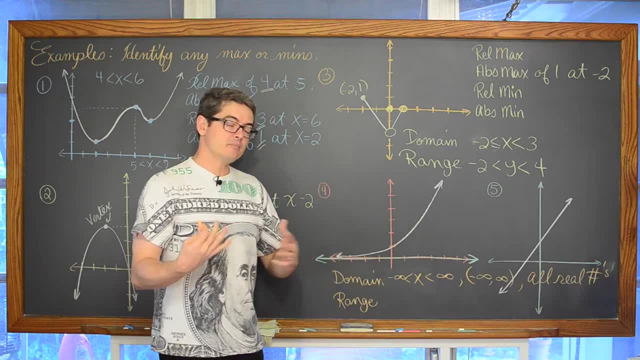 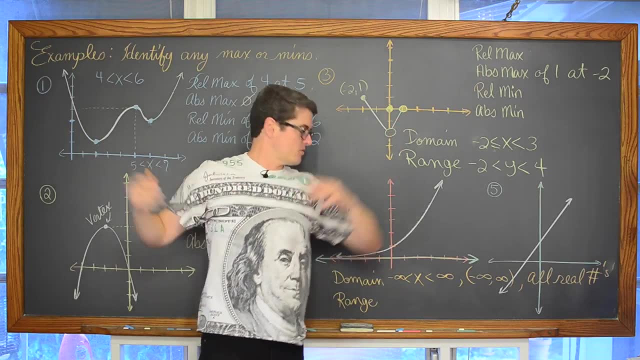 to negative infinity. The range is what we are dealing with when we are identifying max and mens, The y values. What is the lowest y? What is the greatest y? Is it happening on an open interval? Is it the lowest y in the entire domain? Well, the range of this.